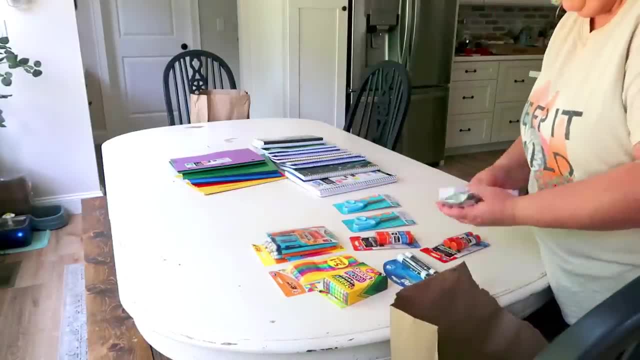 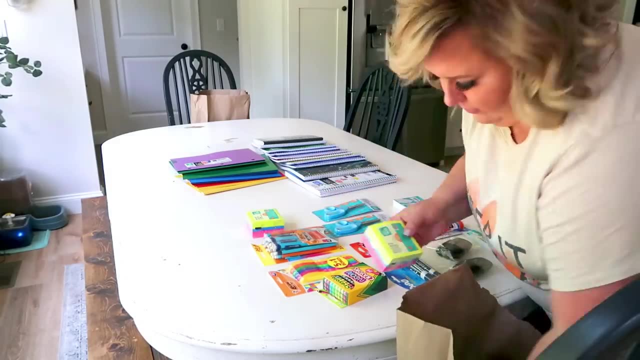 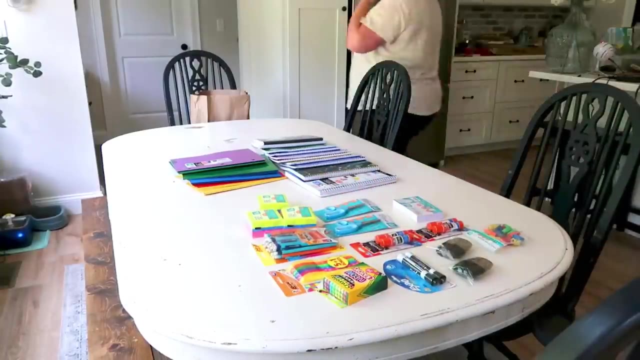 am an elementary school counselor and my husband is a middle school special ed teacher. He works pretty tough and we just love, you know, our summers. but as they start to come to an end, when we start to see the school supplies coming out, we do get a little bit excited too to go back and see. 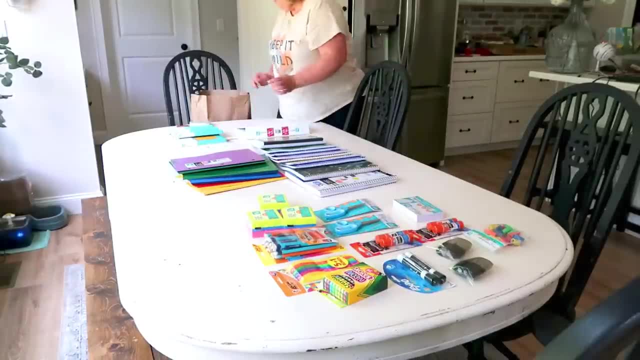 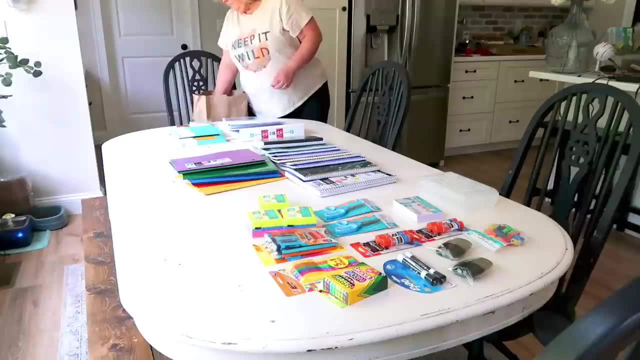 our students. So the way that we do our back to school shopping is we make a list. I take everybody's list and I compile them into one. I use Google Sheets, which I'll show you here in a minute, and if you're following me over on Instagram, I'll talk more about this in my stories today, so you 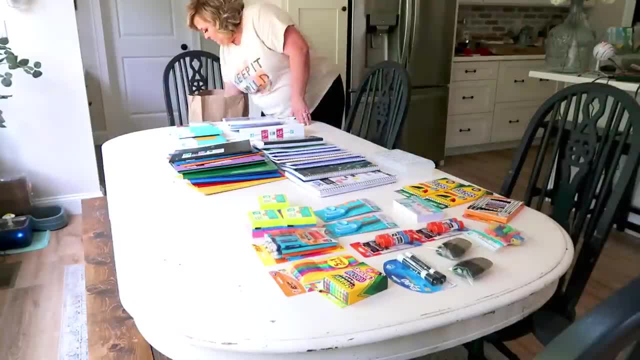 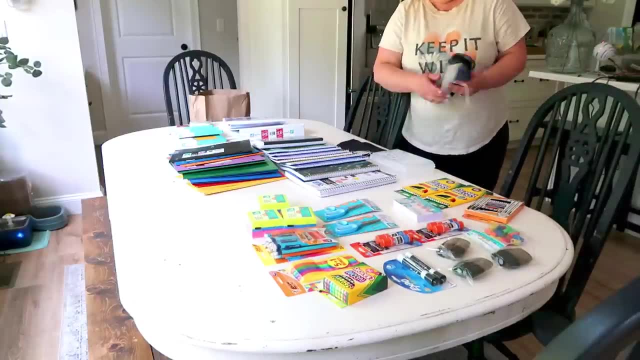 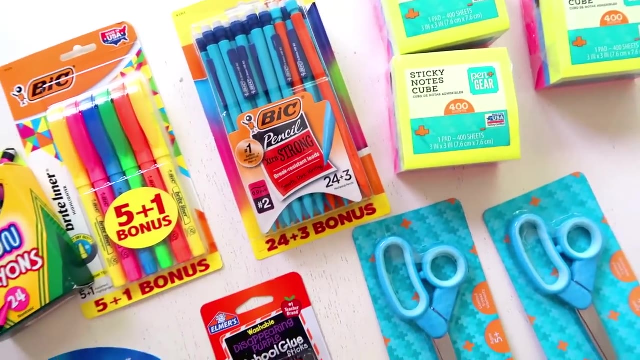 get a better idea of what I'm talking about. But once I have a list that's combined of everybody's supplies, I take that list over to Walmart. Sometimes I do a little bit of shopping over at Target, but 99% of the items I purchased come from Walmart. I just find that they have the best. 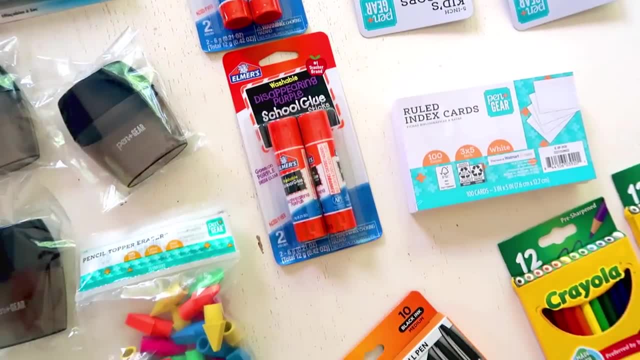 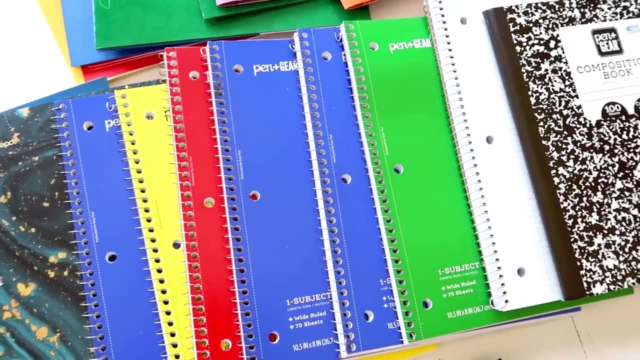 prices for the same exact products. So here's a look at the supplies that I have and these are listed out for my four boys Now, my daughter being in high school, she doesn't get her supply list at school. She also goes to a tech school. She's in a nursing program, so her supply list is a little. 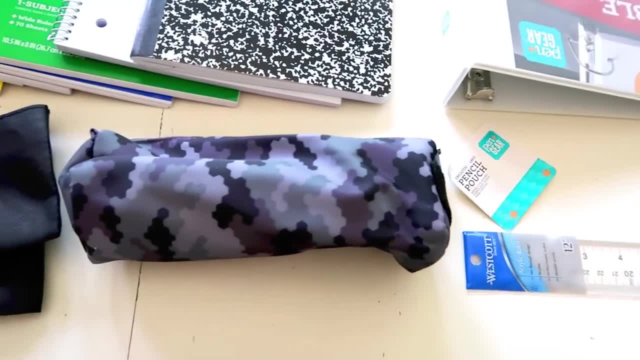 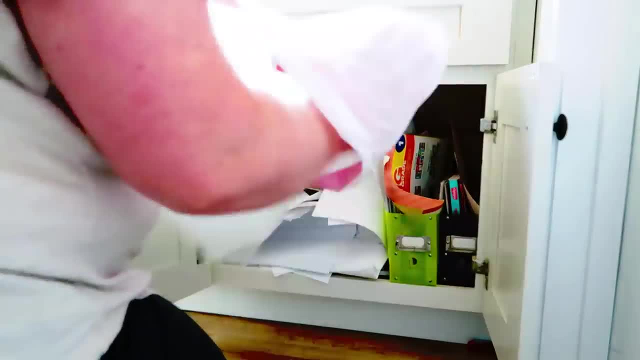 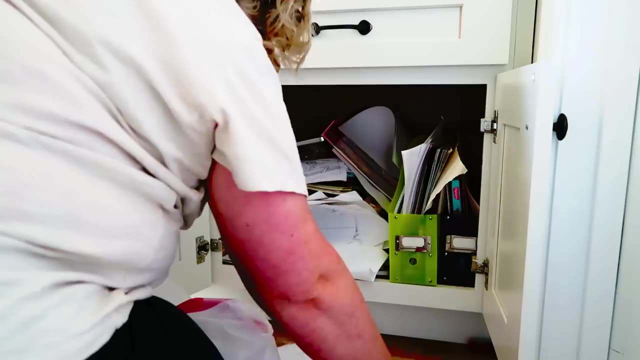 bit different, like scrubs and stethoscopes. So we will do her shopping once she's back at school. but as for the boys, this is what we've got. Next up is this crazy cabinet that I have over in my coffee bar area. As you can see here, it's just been a collect all of rogue papers and pretty much. 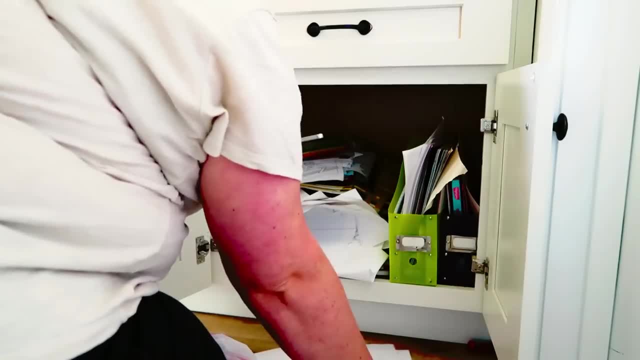 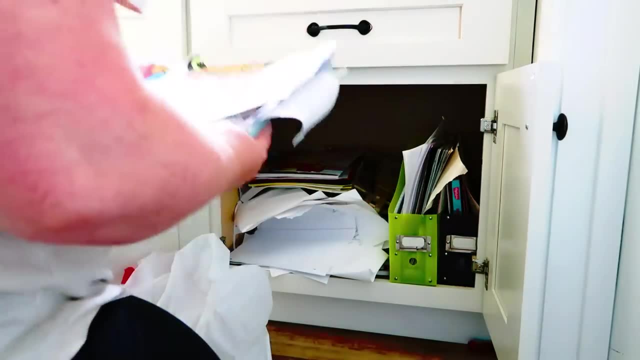 anything else craft or school related. This is where my youngest son, Ryan, will keep all of his drawings. He loves to draw, He loves to color and he's one of those kiddos where you literally can't recycle anything. if he's around, You have. 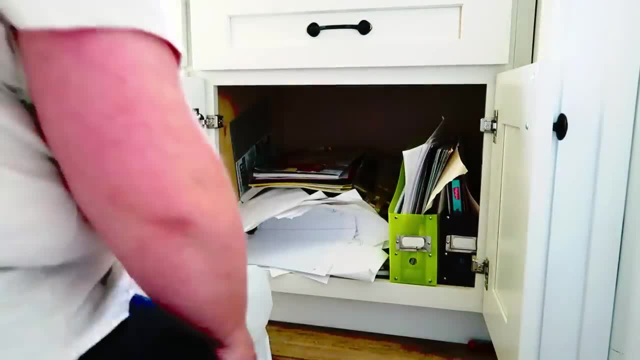 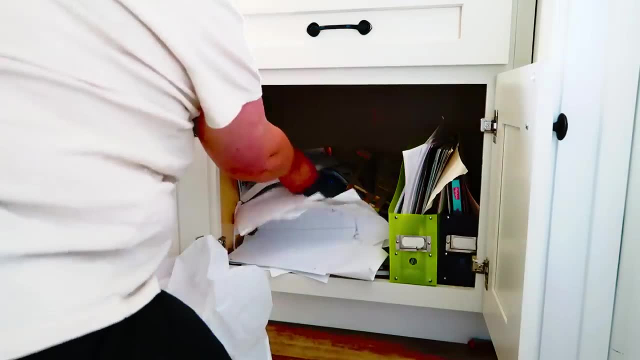 to wait until he goes to bed and then you have to bury it in the recycle bin. That was one of my middle son, Ronan. one of his tests from the school year, He got 100%. These are the things your kids just don't want to get rid of. and I do have one of those cool, you know filing cabinets where you 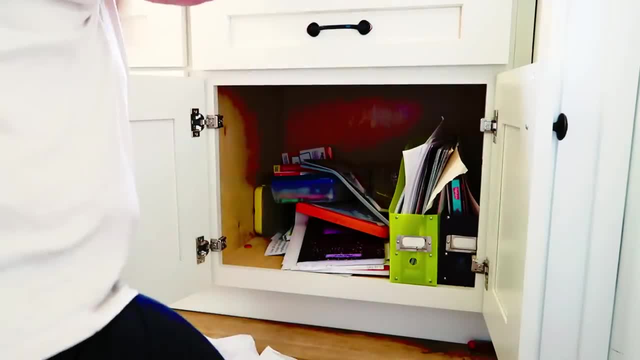 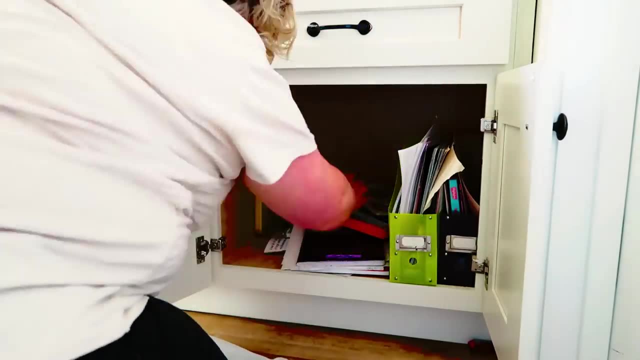 keep some good keepsakes, but I can't keep them, So I'm just going to keep them. I'm going to keep everything you guys. It's just not feasible. So I know there's lots of fun ways of taking pictures and making a book that way and all that good stuff, but we're going to get all of these things out of. 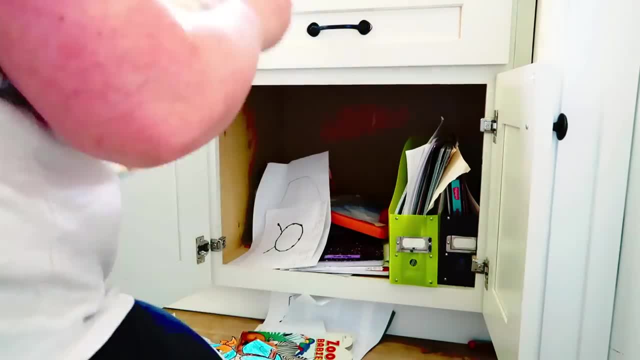 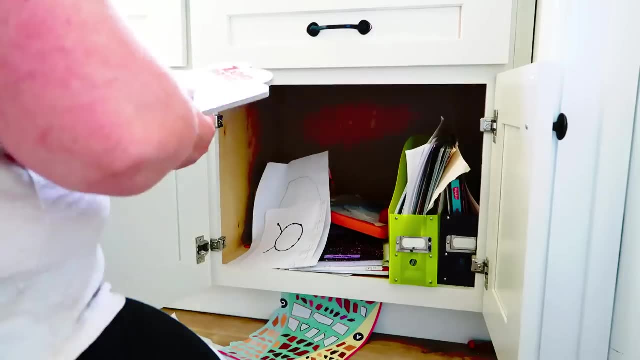 here and then we're going to figure out what it is we're keeping and what it is we're getting rid of. So there's sticker book stuff in here. There's regular books in here, Coloring books, tracing books, all kinds of stuff in here. but I wanted this to be functional before you go back to school. 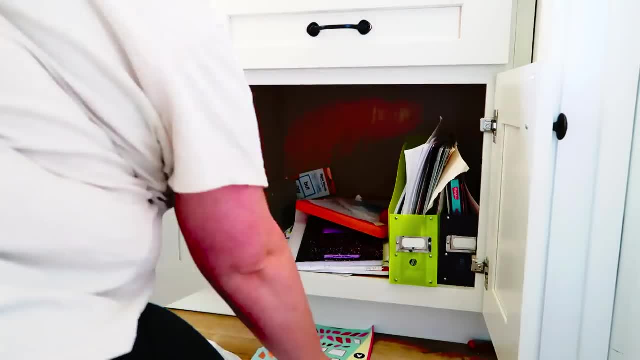 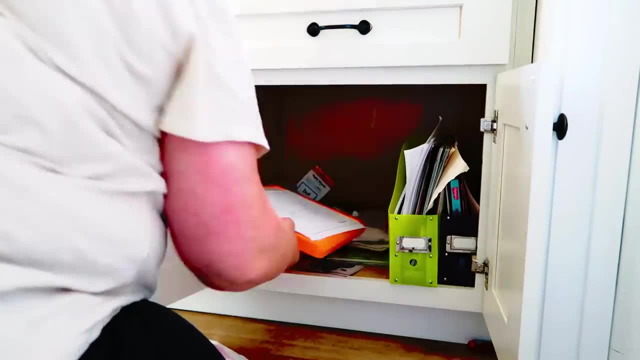 This is also where loose leaf paper will be kept, and these are things that they'll need for when they're working on projects at home. So, like I said, I needed it to be organized before we started the school year, and it needed to be done. I had just. 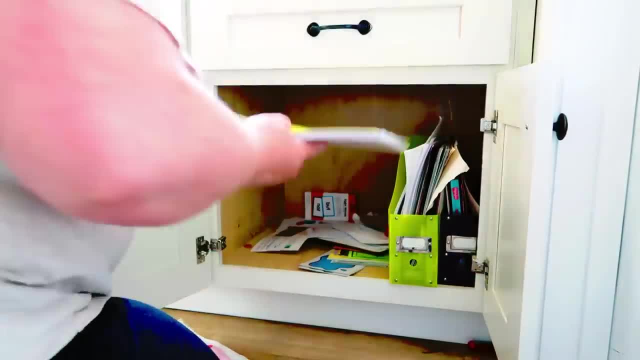 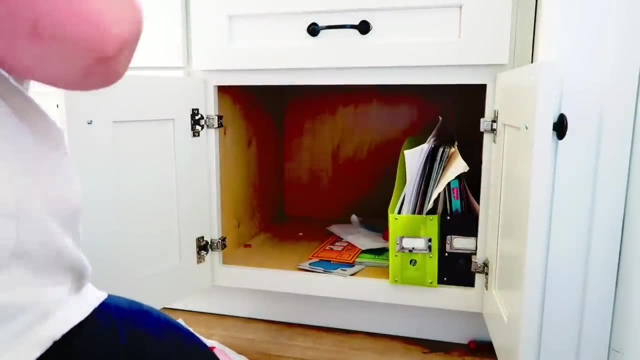 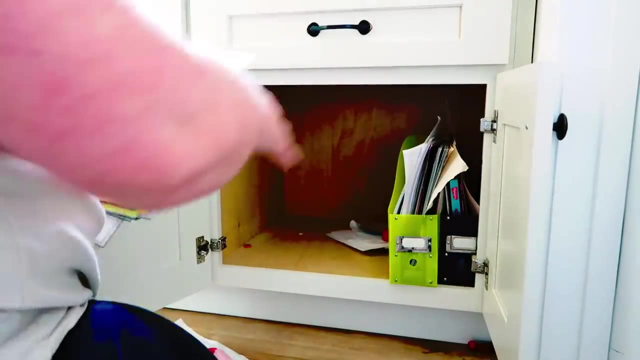 been putting it off for so long. So I'm just going to remove everything from this space here. It's pretty small, but it was really deep and, shockingly, there was a ton of stuff in here and I hadn't done this since we moved into the house. I didn't even really organize this space, I just kind of tossed. 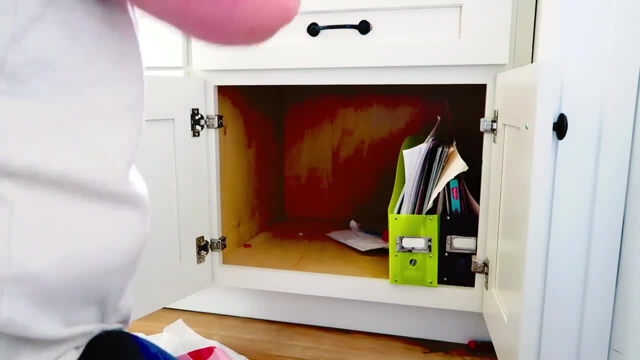 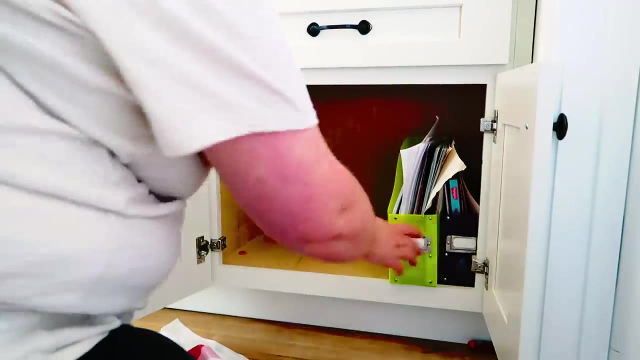 stuff in here, So this is what I'm working with. right here in my hand are the schedules that we used when we were doing home- not homeschooling, but remote learning. The little tasks were on velcro so I would move them around every day. My kids all had one and they'd have to check off what they did, and that's. 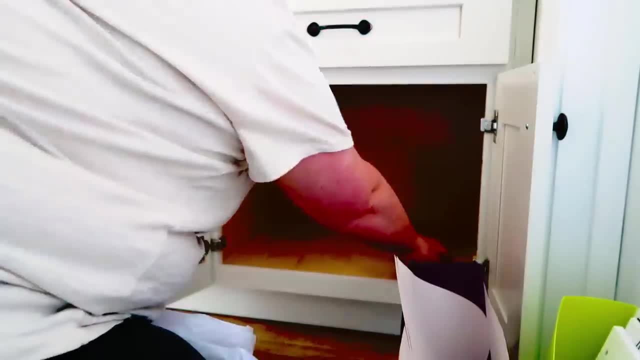 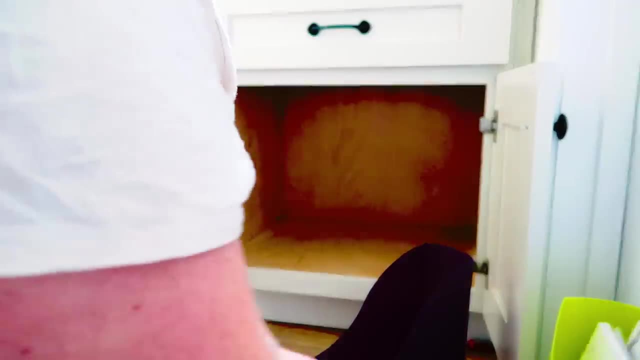 because they did remote learning with my mother-in-law while I was at school, So it was just crazy That was while we were doing hybrid learning. Isn't that nuts to remember? like to think back to what that was actually like, Like we actually did that and lived like that for a little while. I'm glad that's. 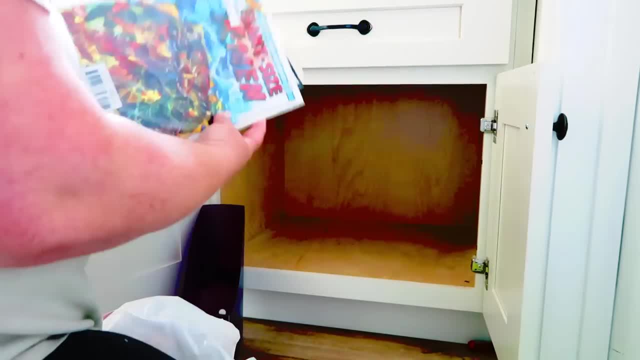 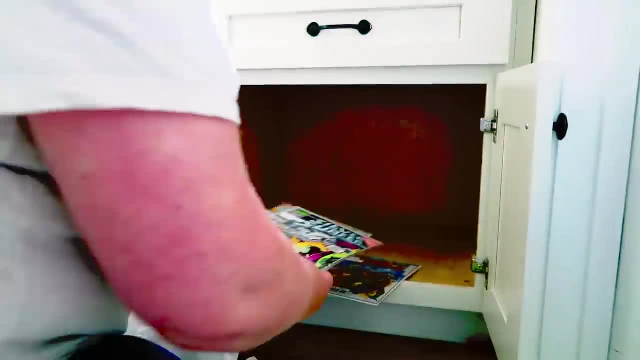 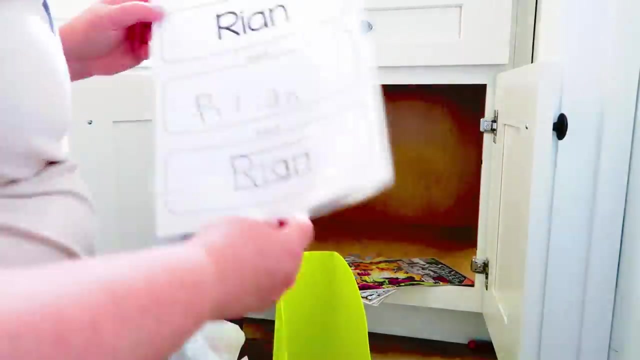 over. Well, at least that part of it anyway. So now I'm just kind of going through the books, the comic books, the coloring books, all of that other stuff, deciding what it is that we're going to keep, and then I'm going to clean out this entire area and then we're going to get to organizing. By the time, 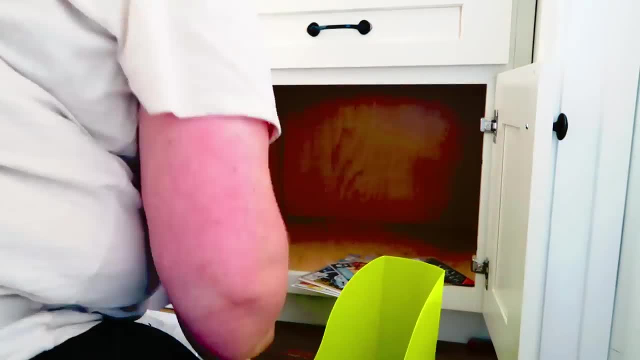 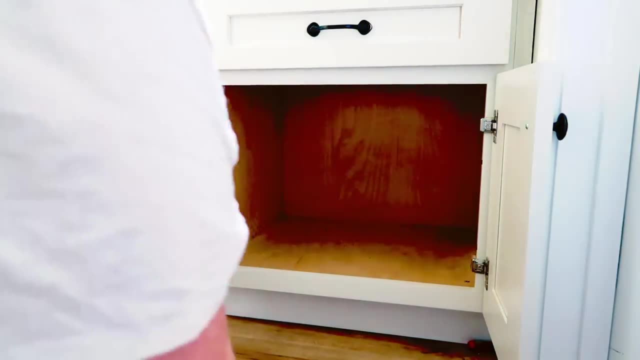 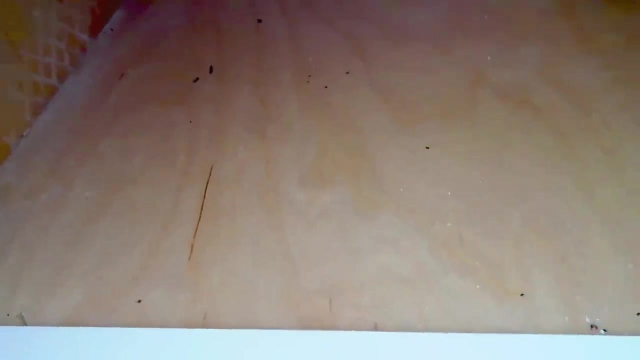 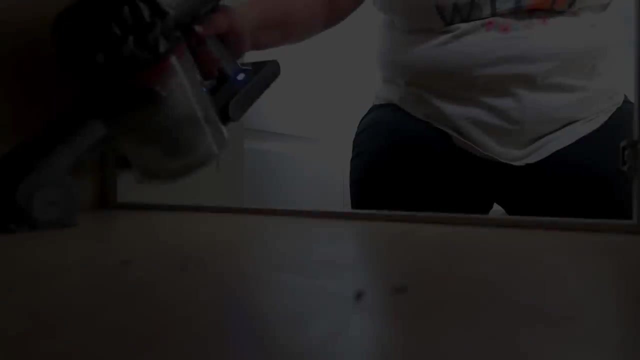 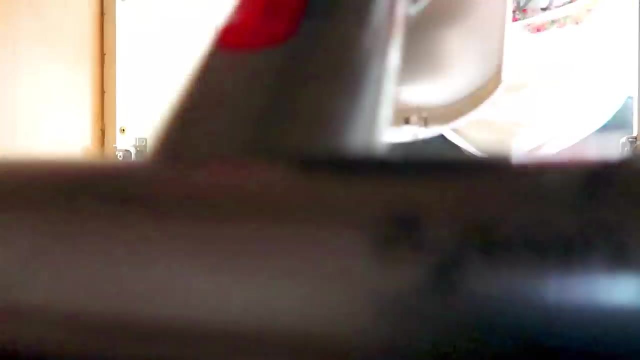 we're done with this. it'll look, you know the way it's supposed to- Just using my vacuum real quick to vacuum out all of these wood chips. I think I don't remember vacuuming out the cabinet before I put everything in, So I'm just going to vacuum out all of these. 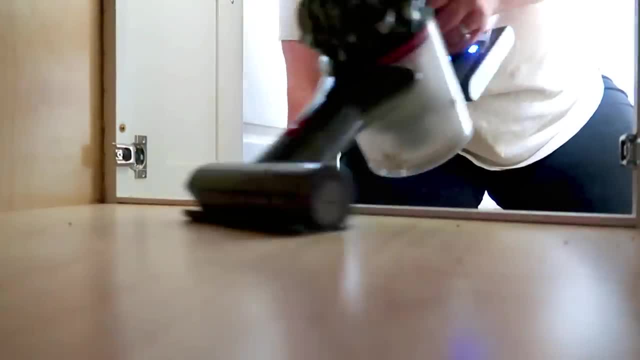 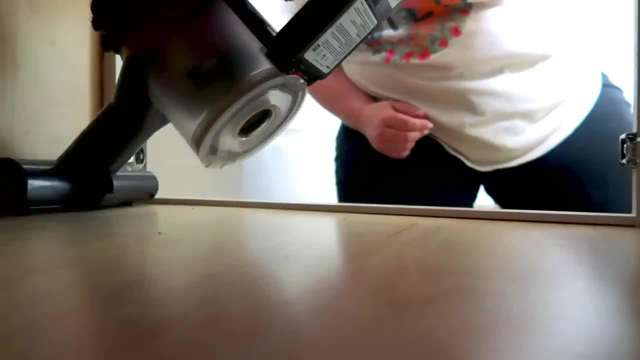 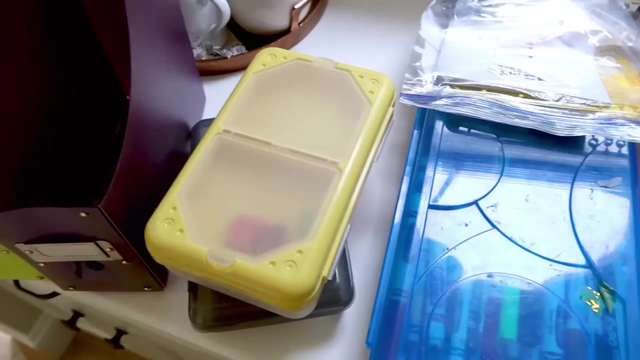 things in it. So there was a little bit of wood chips from when they screwed these into the wall, the cabinets into the wall. So just getting that cleaned out real quick and then we're going to get the items put back in nicely, So really quickly. I'm showing you this is what I kept. 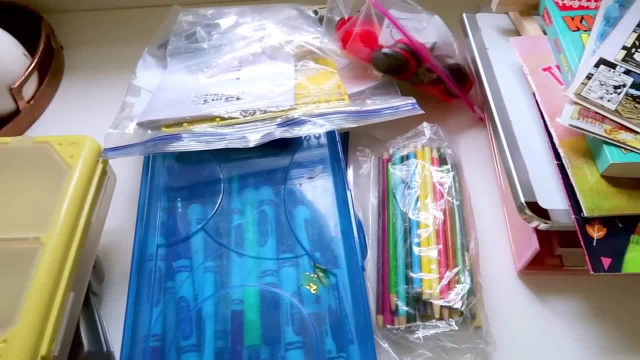 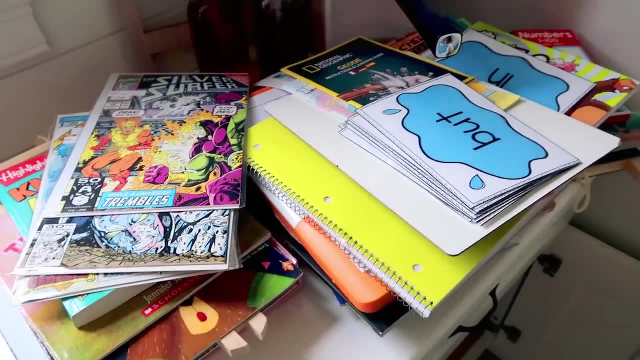 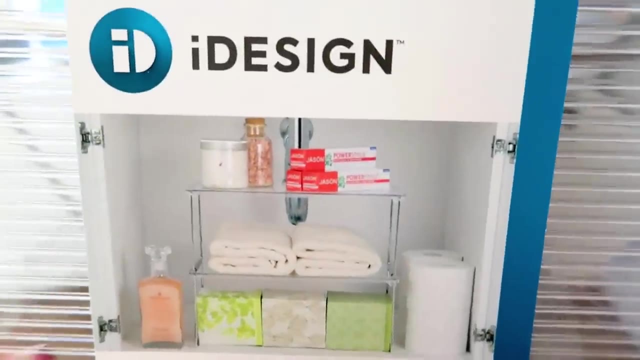 out of all of those things you saw me pull out of there. So much stuff I pulled out and this is what we're keeping, So it's not really a ton. It's just the important stuff, like sight words and coloring books, and we're going to start by using this stacking shelf. I purchased this at Walmart. 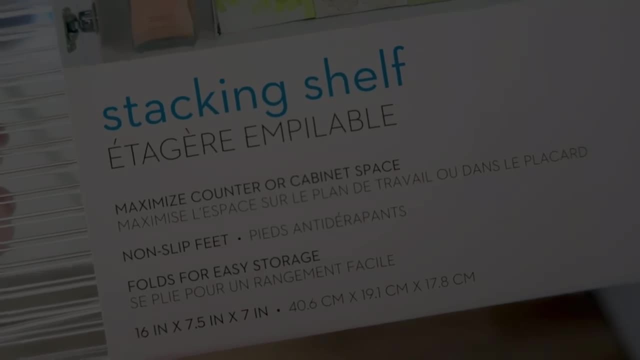 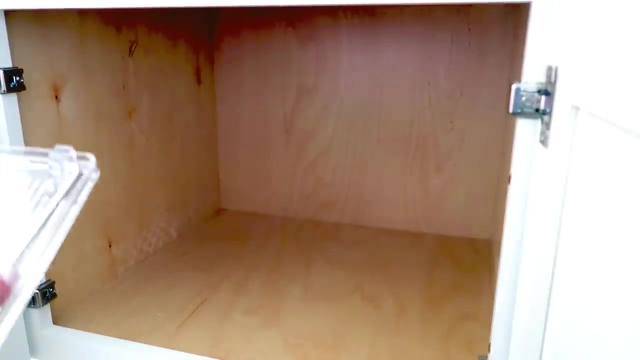 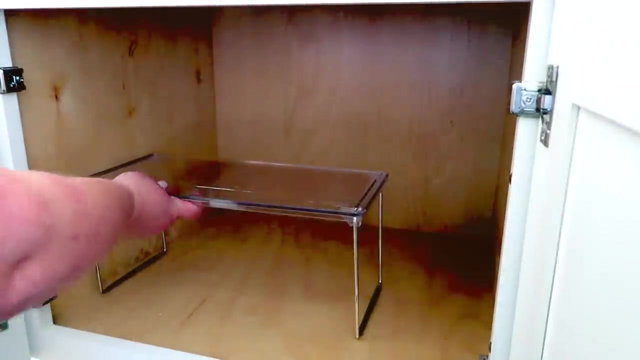 I want to say maybe for around seven dollars. I'll try to link it for you down below, but it's just a little clear plastic stacking shelf. You can, you know, stack two on top of each other, but I just needed one, because the cabinets that we chose for over here didn't have any kind of shelf. Now we 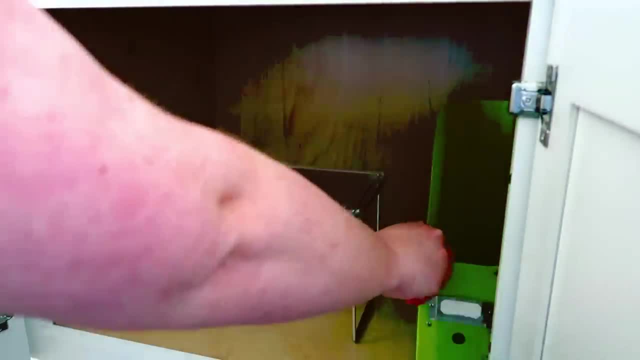 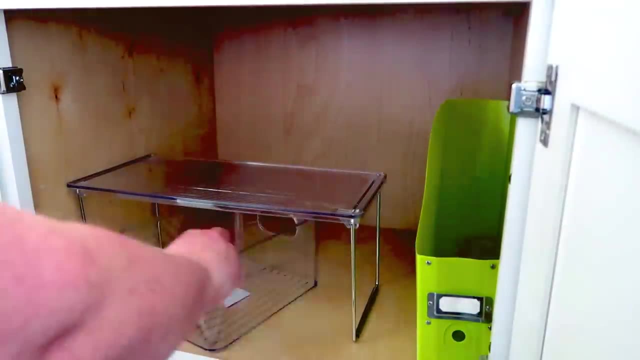 purchased these cabinets from cabinetscom. These are the exact same cabinets that we chose for over here. These are the exact same cabinets as our kitchen. however, to keep them a little bit more cost affordable, We went with no shelf, and I deeply regret that. I wish that we had done some kind. 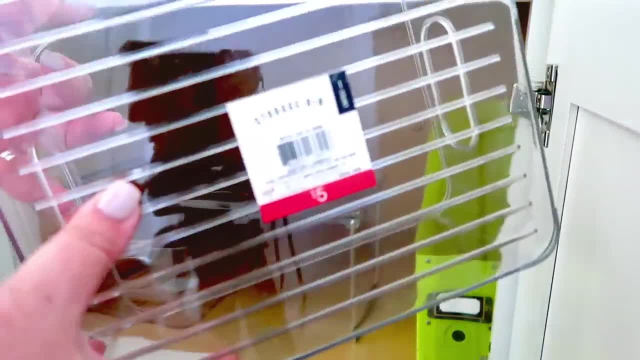 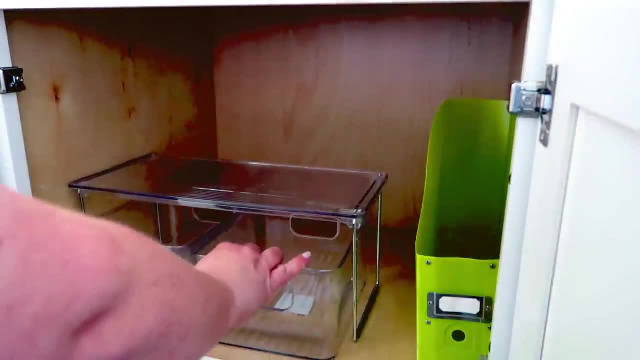 of pullout shelf like we have in our pantry. but that's okay, We're going to make it work. We're using these five dollar storage bins that I found at Target in the dollar section. They feel almost identical to the home edit ones you find at Walmart, but they were much, much cheaper. 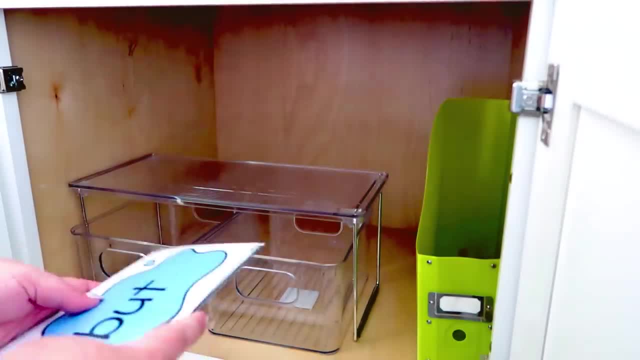 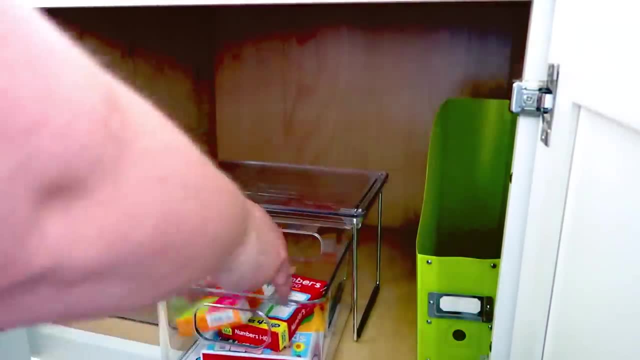 and they were readily available. So I grabbed two of those slide right under the little shelf right there and in the first one, this is where I'm going to keep all of our flash cards. We have sight word flash cards and you know, I just I think they're all. 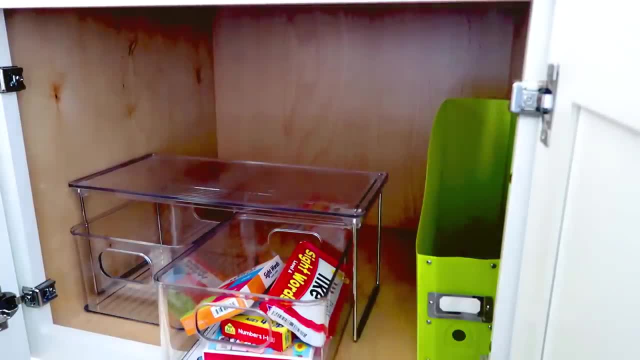 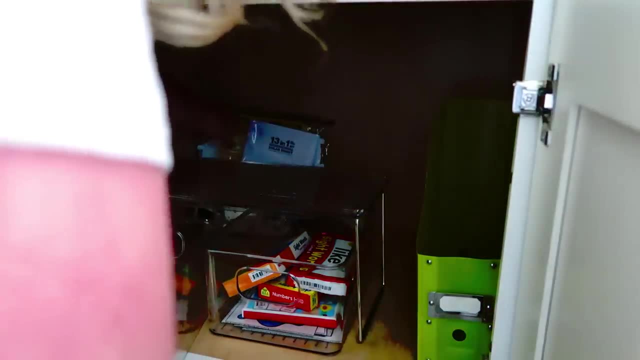 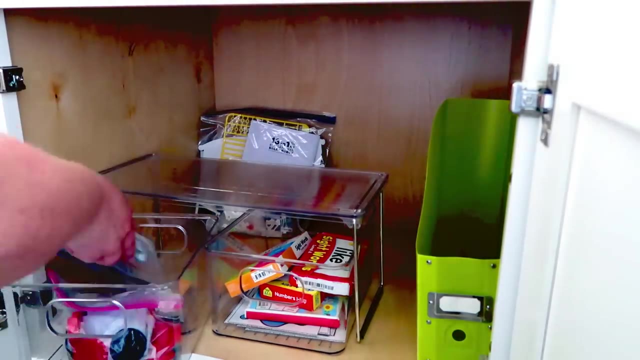 reading flash cards. So we're just putting all of those there in that drawer so they're easy to find. and then in the other one- I think I just got started with some games, but I do end up moving those things around- I've got a checkers game there and then I think I also put in a bag of our 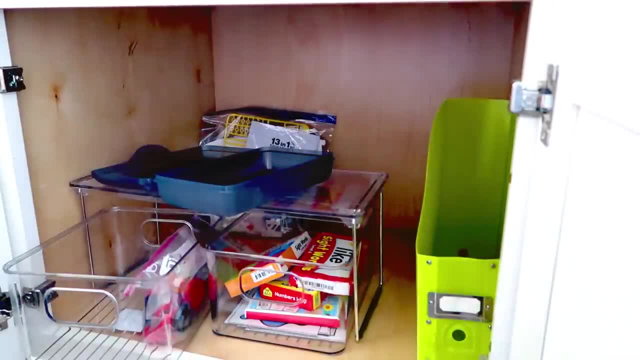 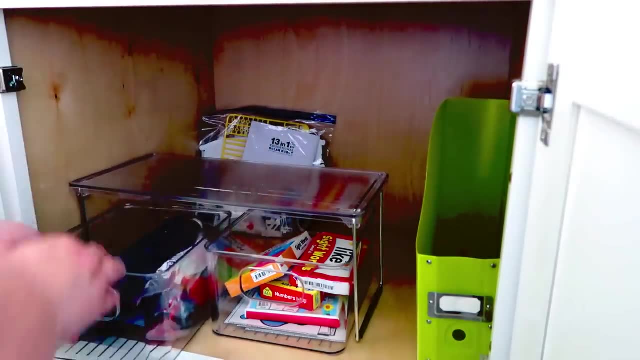 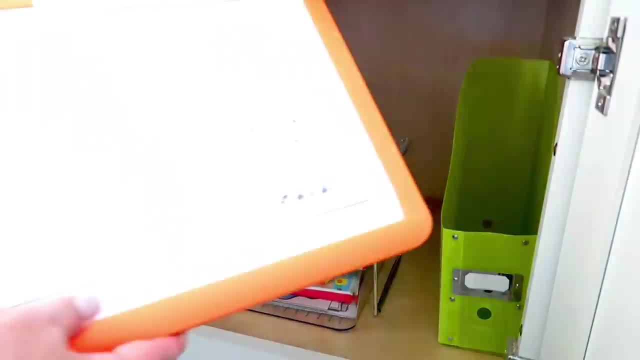 those are colored pencils that we use like on the go, kind of like grab and go outside, grab and go in the car. but I decided to put them into that pencil box, which those, by the way. I have so many of them, but they're 97 cents at Walmart, so really good to have on hand. Then we have this tracing: 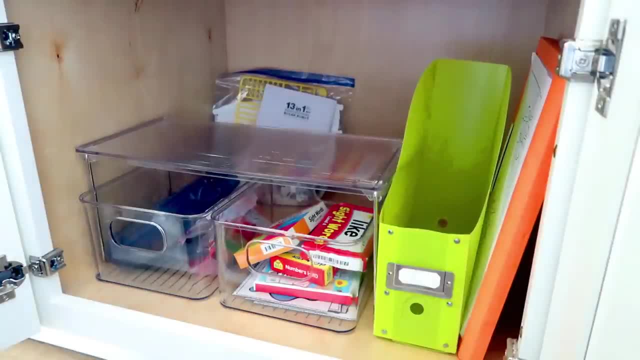 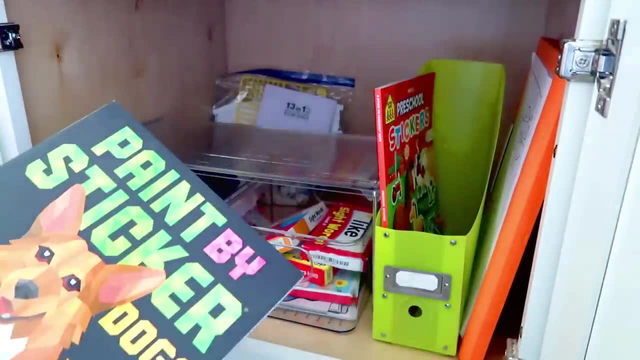 board clipboard. I'm not really sure what you would call this, but it lights up. Ryan got it for Christmas last year and he loves it. you can print any picture, stick it on there and then it lights up and you can trace it. We also have a lot of paint by sticker books. you can get these on Amazon. 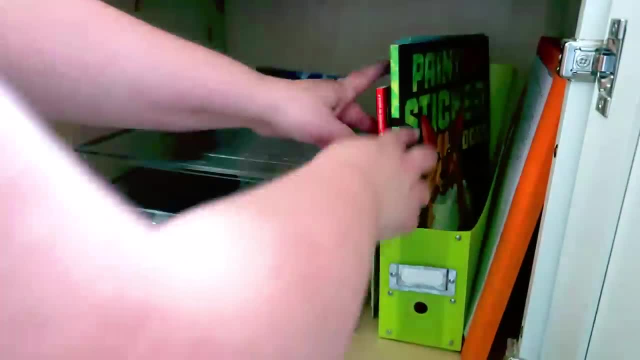 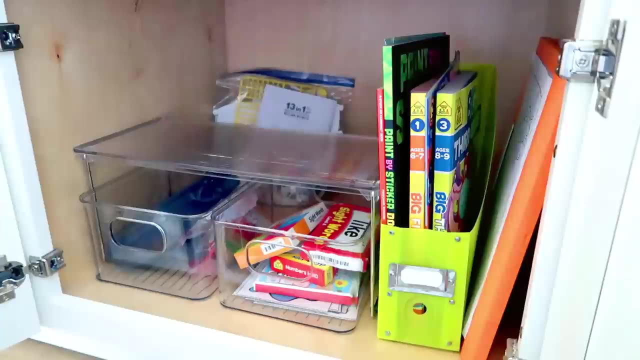 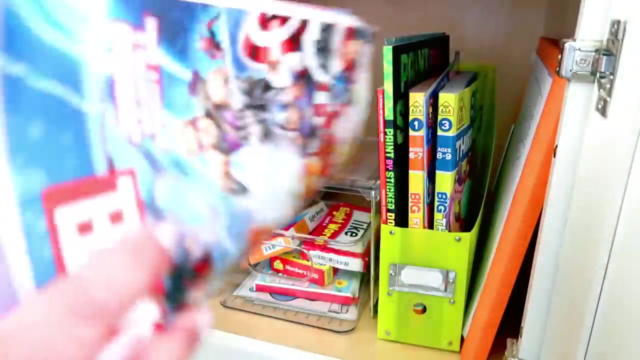 I have also found them at the Dollar Tree. not those really big, nice ones, but I have found some at the Dollar Tree. those are really great activities for your kiddos if they just need something to do that's calm and quiet. They're good for rainy days. they're just really good to have on hand. they're good for adults too. I. 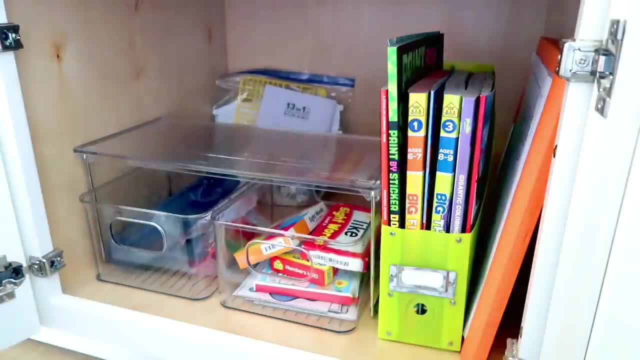 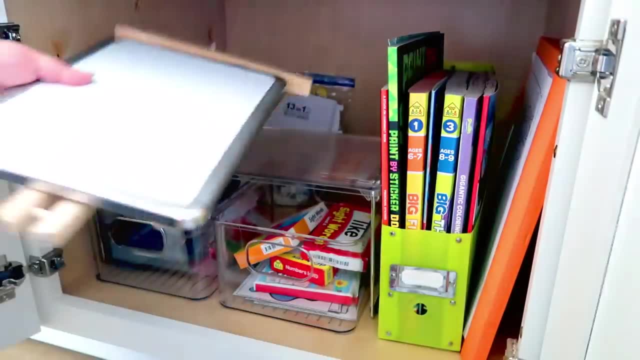 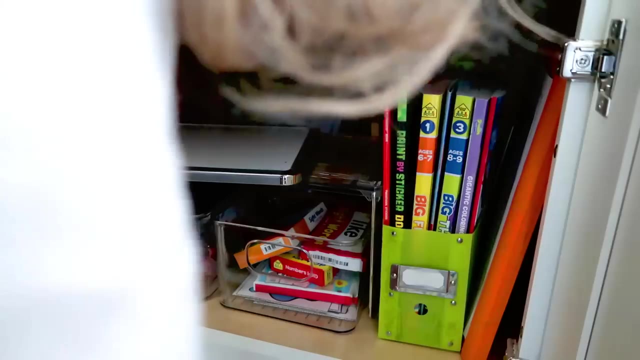 use them too. and then we just have regular coloring books and just some workbooks. so putting those all into just like a like a paper collector- I don't even know what kind of organizer you would call that- and then there's an easel with a whiteboard- which you know random, but 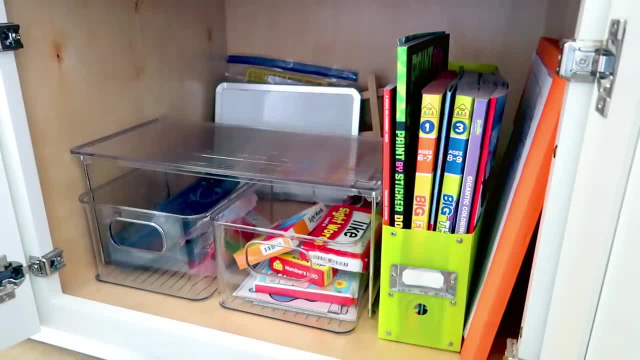 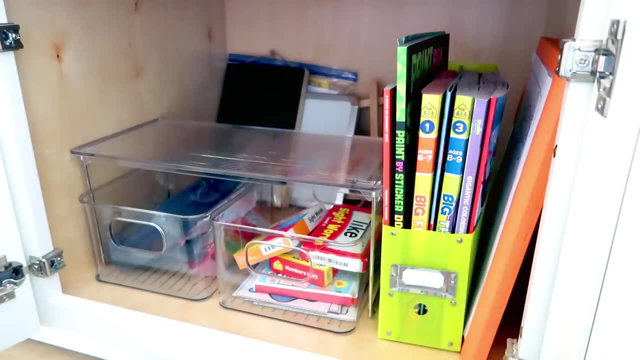 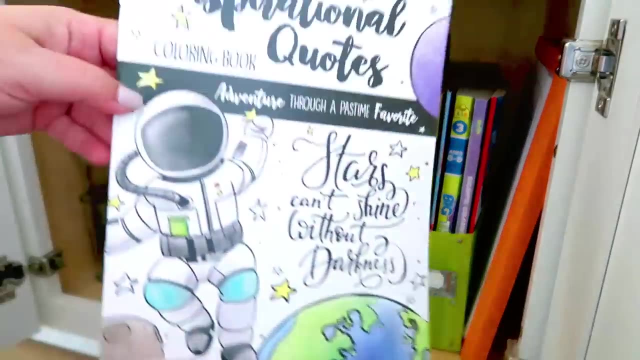 it's kind of things you have When you're both an educator and you got a bunch of kids. we also have a chalkboard easel, which on the other side is a whiteboard, and then I also was just grabbing whatever was on top up there and finding a home for it. so here's another coloring book that is, you know, more for adults. 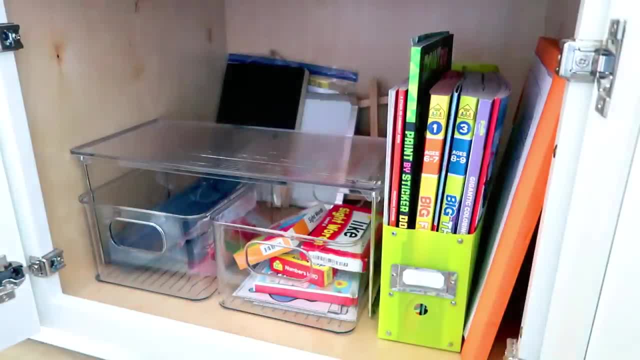 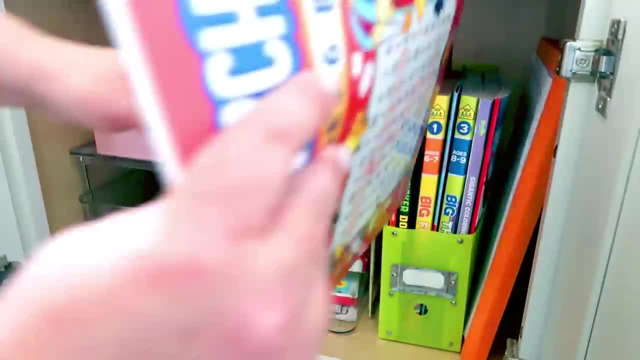 found that at the Dollar Tree. by the way, it's got really sweet, like inspirational quotes inside. that's the one Michaela loves to use. so I also found this paper holder at the Dollar Tree, and so I'm just putting that on top of that shelf now. obviously, the paper holder is a little 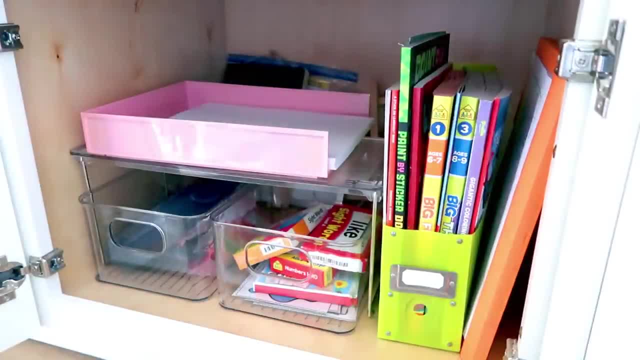 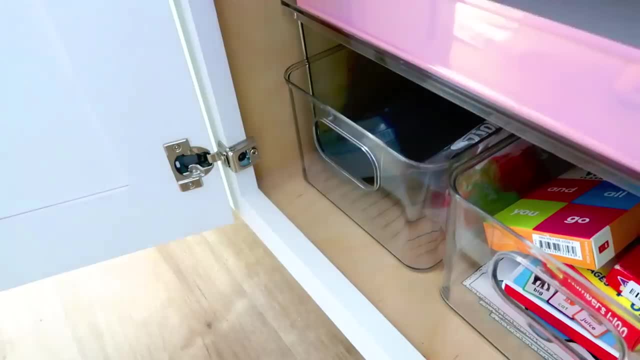 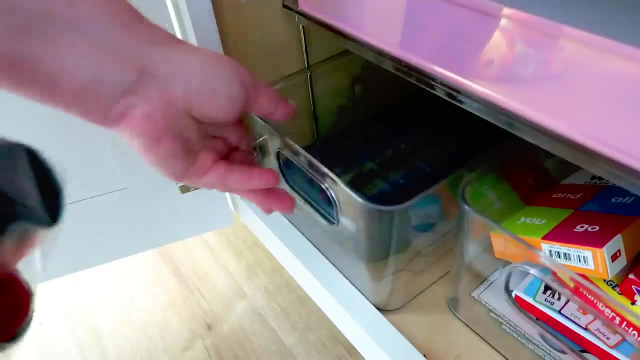 bit wider than the shelf but it works perfectly fine and I'm adding in some just really cheap printer paper that Ryan uses to draw and color on and then in this container here. I decided to kind of rearrange things because I wanted to add in some books, so I'm moving the game here. 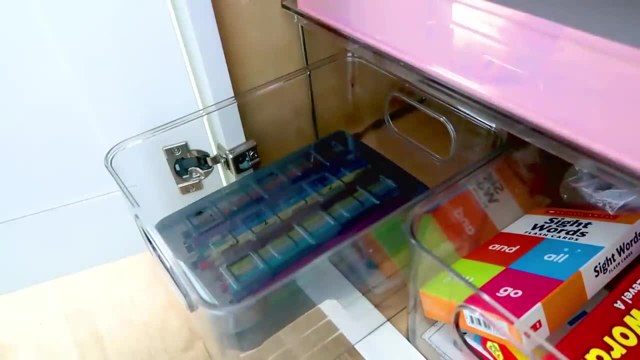 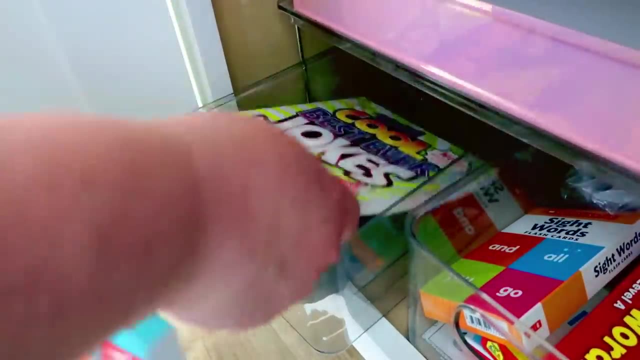 the chess game into the back, Where the books are- I'm sorry, where the sight words are- and then I'm adding in the kids joke books down here when they need to read, but they don't want to joke. books are always the way to go because it's easy for them to read them out loud. so if you're cooking dinner and you need your kids, 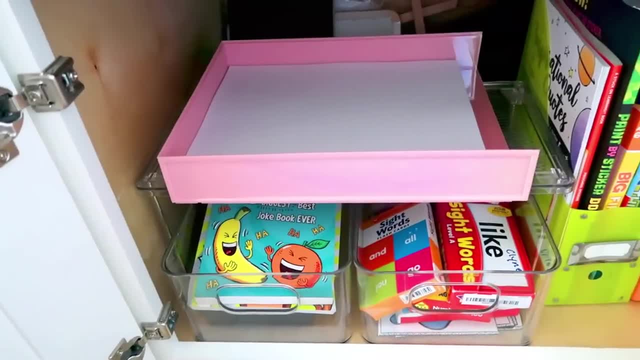 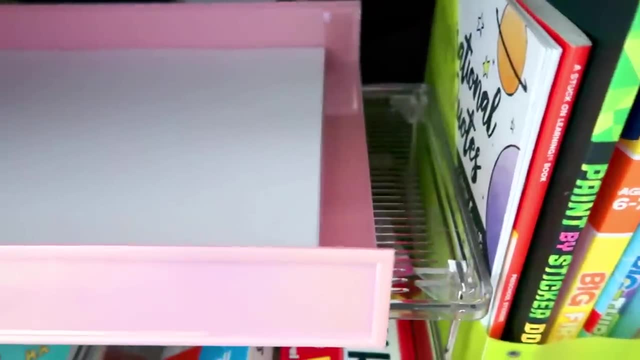 to get some reading in. grab a joke book and have them read them to you while you're cooking or doing some chores around the house. so here's how that crazy cabinet turned out. it's crazy to think of what it looked like when we first got started. this is definitely much, much more functional and 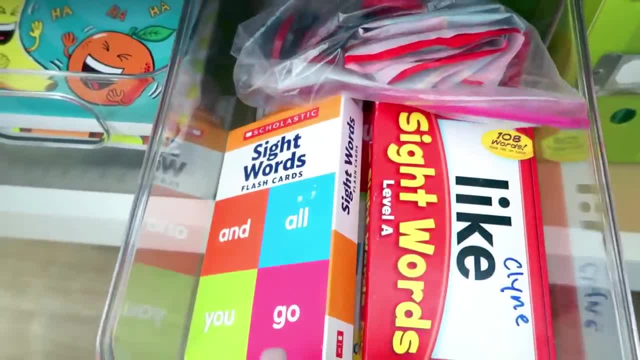 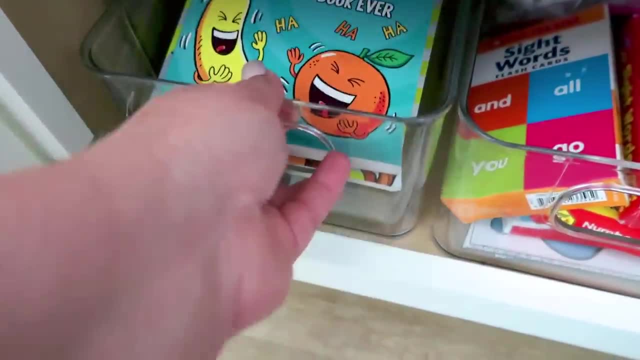 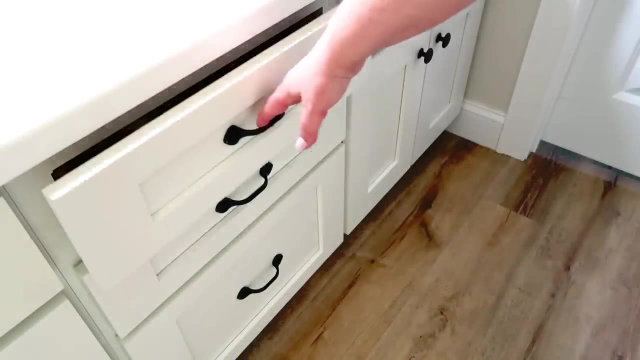 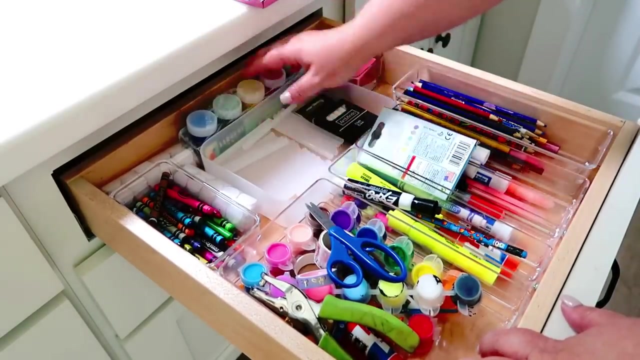 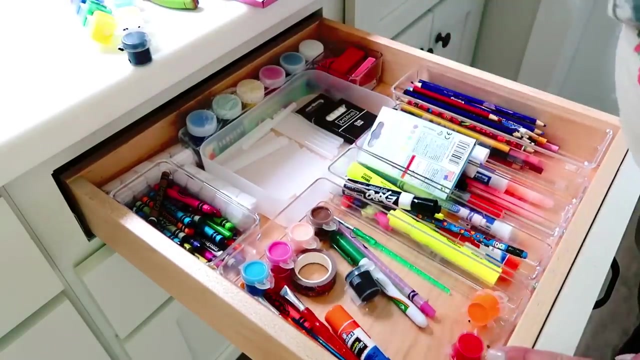 it's going to be a lot better when we go back to school- way less headache. next up we're going to work on our supply drawer. so I do have a video of me organizing this the first time in my coffee bar- organize and decorate video. I'll have it linked for you down below, but in this video we're going to actually clean it out. so 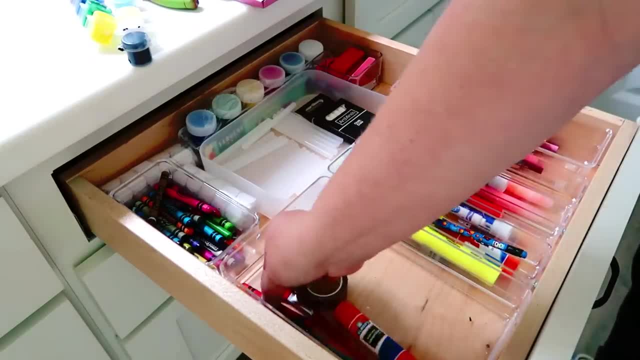 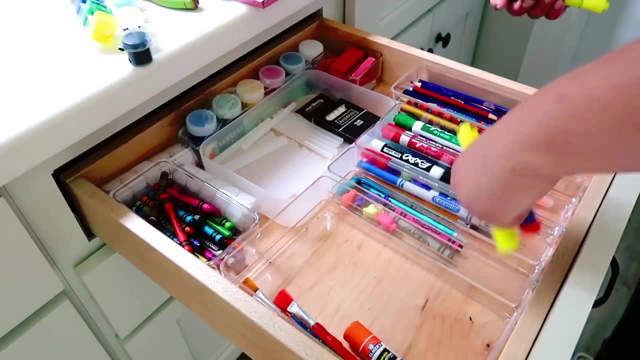 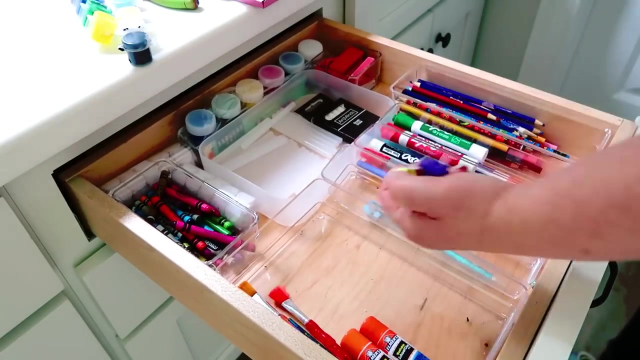 this gets used every single day. my kids love to do arts and crafts. they're in here all the time. my mom is actually visiting from Colorado right now and they've been doing tons of craft activities yesterday. yesterday, they made really cool journals with felt covers, um, so they're just. 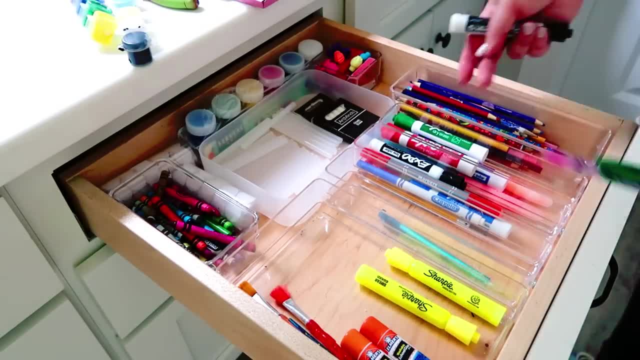 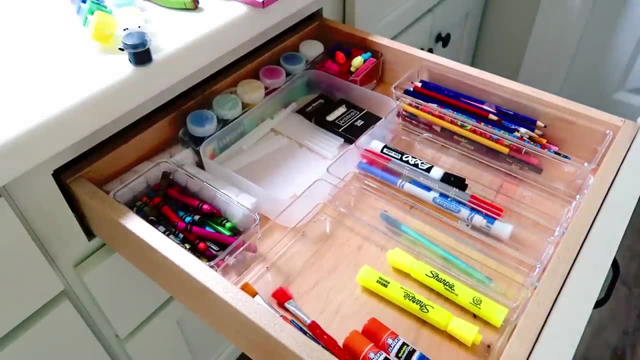 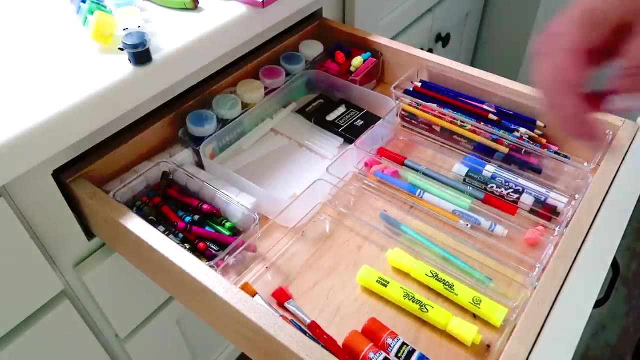 you know, we're always in this drawer. my kids are very, very, very um artistic and creative, so it's gotten a little messy. uh, since I, you know, organized this back in January, so we're going to get it reorganized, I'm just kind of moving things around and finding things that I know they're going. 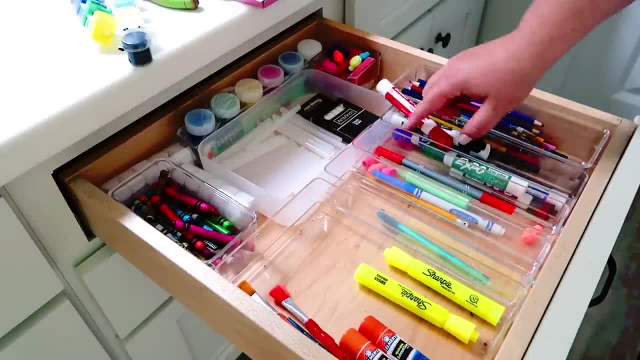 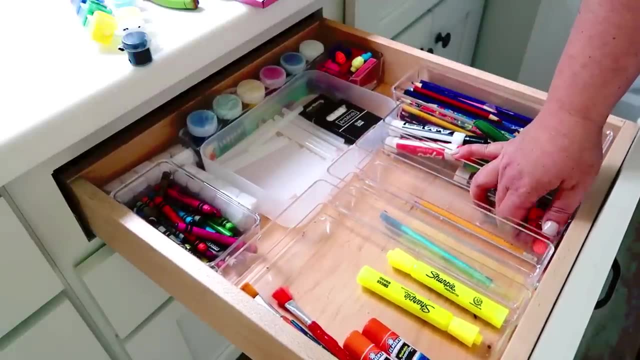 to need for homework and for studying and making sure we have those, like those dry erase markers that I'm doing right there. we've got some fine tip markers we're going to bring in. I'm also removing old, um, you know, kind of dried up items and I'm going to replace them with new, fresh items for this. 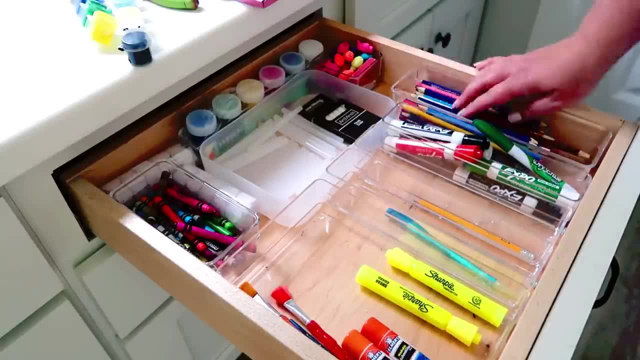 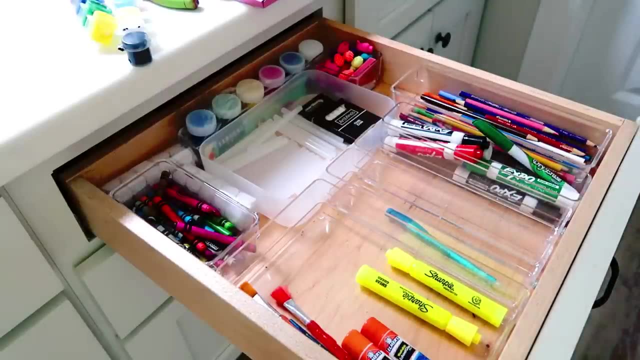 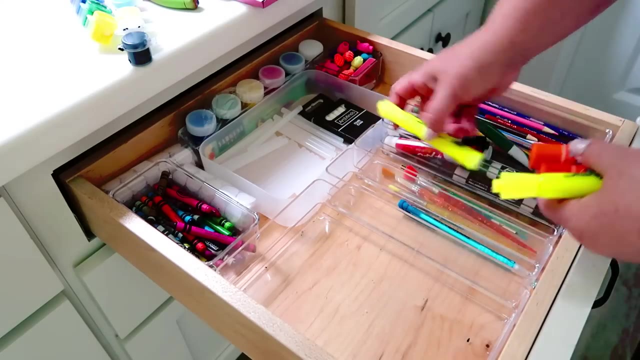 school year. and what happens is when we do have older items that aren't all the way done yet and there stays still some life in them, they go into our travel um pencil case. so that travel pencil case you saw with all those coloring pencils, I'll put some markers in there and that way you know. 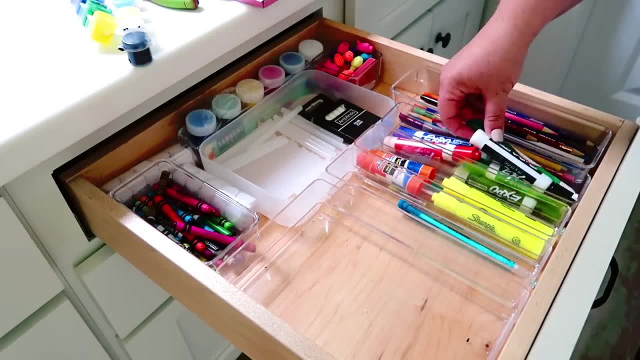 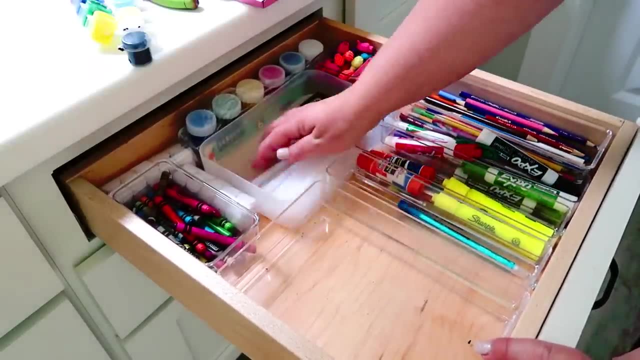 they can take that with them outside. they love to take a blanket outside to the front yard, um, but I'm not getting rid of them. they're just coming out of here because this is what we're going to use, you know, for back to school, for homework and for school. so I'm going to get rid of them and I'm going to 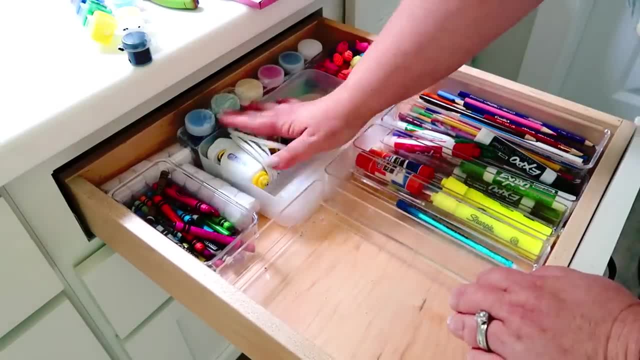 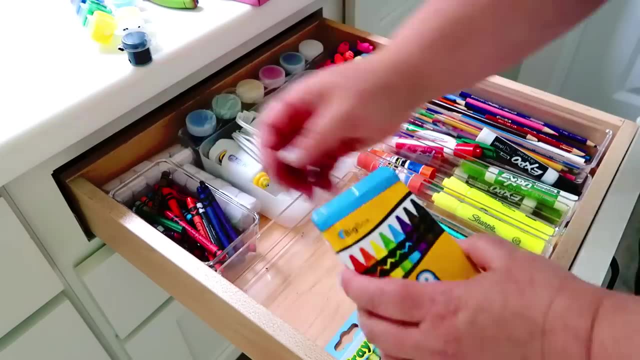 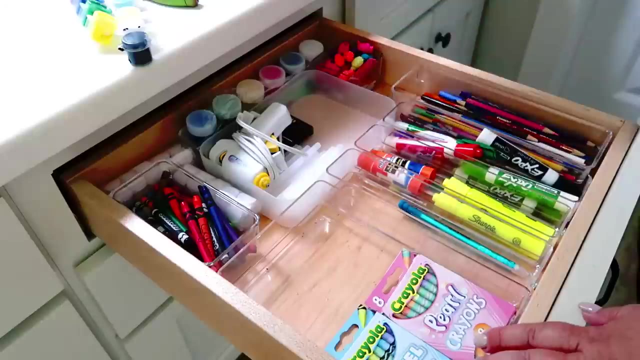 homework and projects, So we're going to kind of just move things around. Now. the containers that I have in this drawer are from a couple of different places, So the clear containers are from Amazon, and then the white container in the back, where the hot glue gun is, that one is from. 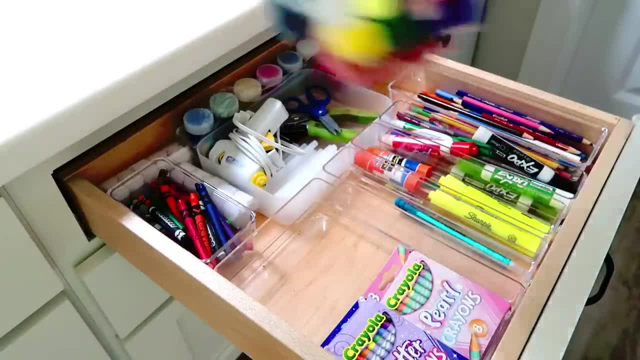 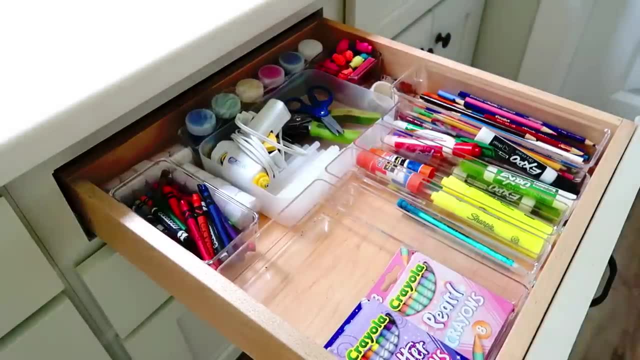 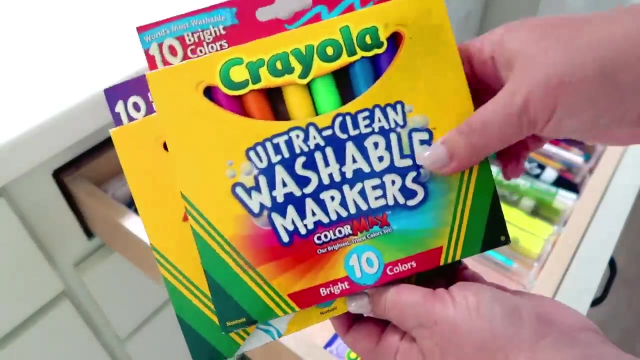 Target, Trying to think if there's anywhere else. I think that's the only two places where I purchased these, but I'll try to link them. I do believe the thinner containers are or the clear ones. I'm sorry, are actually already linked in my Amazon storefront, But if you can't find them, 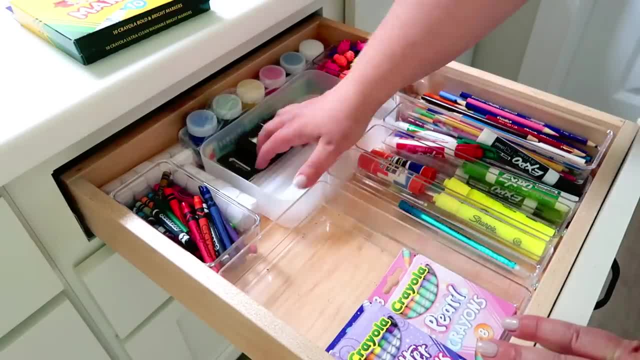 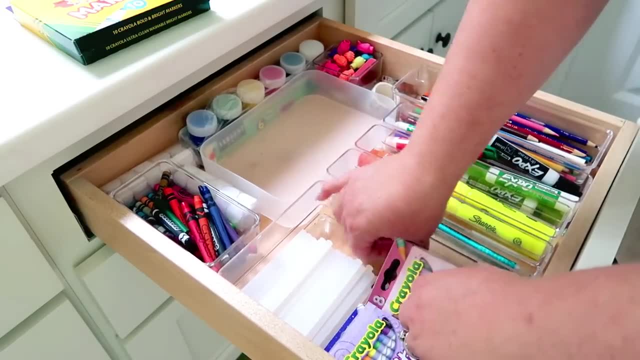 just let me know and I'll find them for you. So just going to go ahead and kind of rearrange things, move things around as much as I can, try to get everything to fit the best way, And I love the way this drawer turned out. There is nothing more satisfying than opening up this drawer and 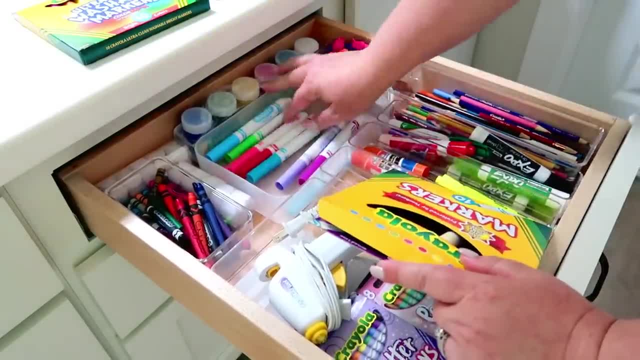 seeing all of the things that I have in here, So I'm going to go ahead and open this drawer and all of the color, so neatly organized, It just turns out really beautiful, So I'm excited for you to see how it turns out. 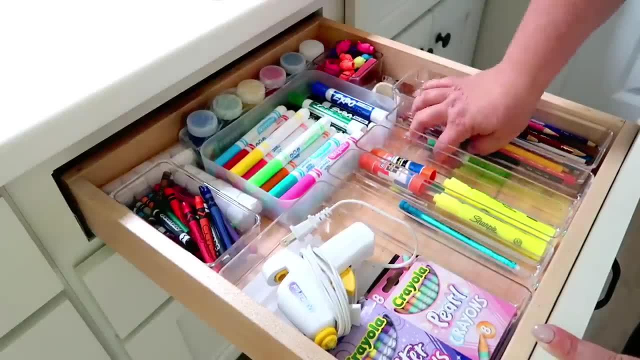 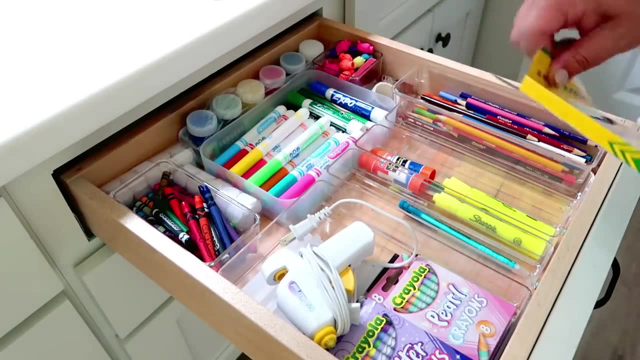 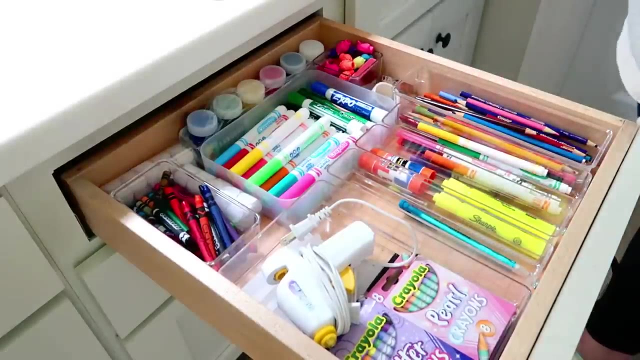 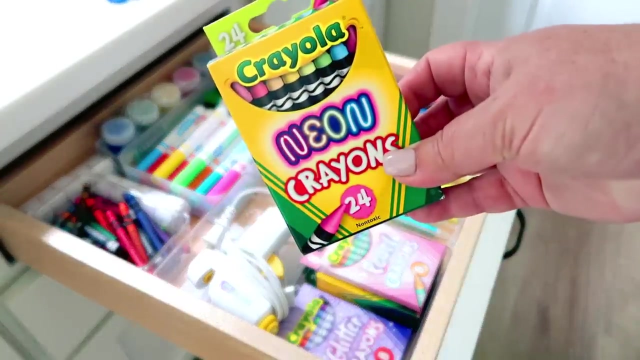 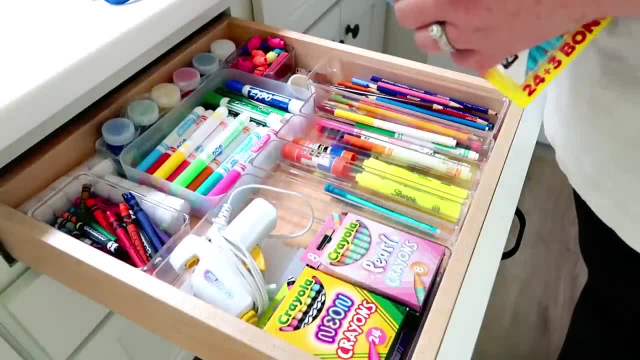 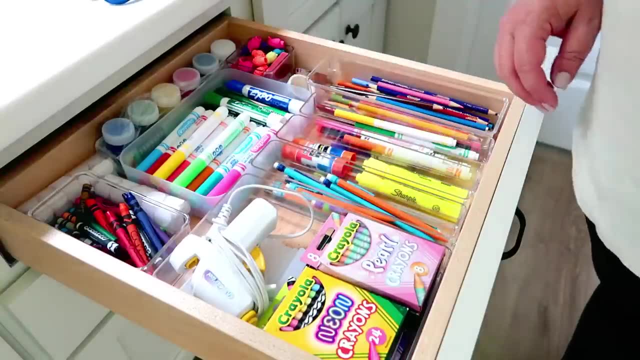 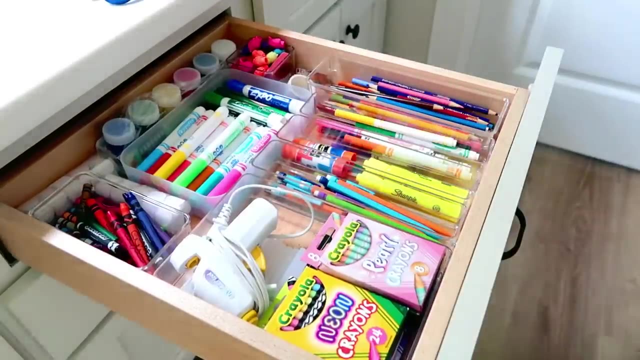 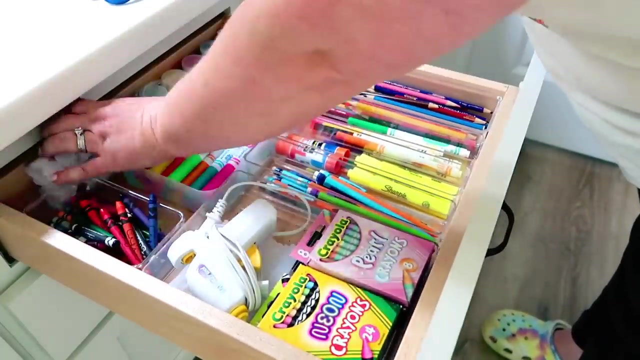 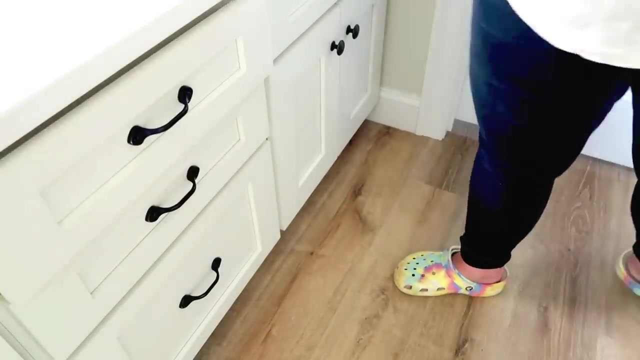 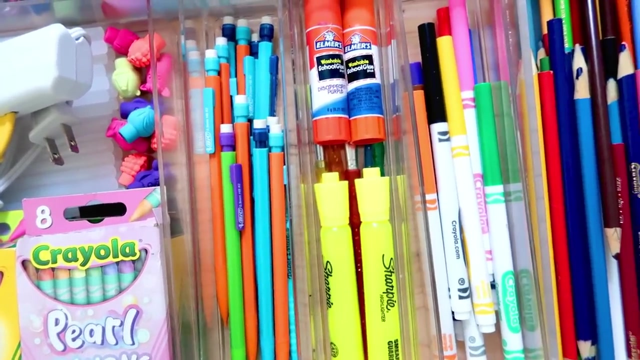 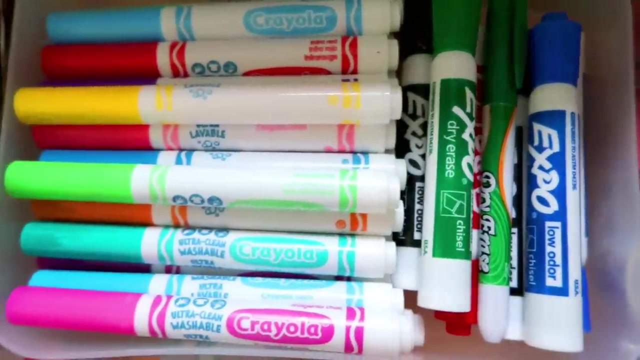 Thank you for watching. And here is the final look at the supply drawer. I love how this turned out. There is nothing more satisfying than a bunch of back to school supplies all neatly organized in a drawer. We're ready. We're ready for your school year. Let's bring it on. 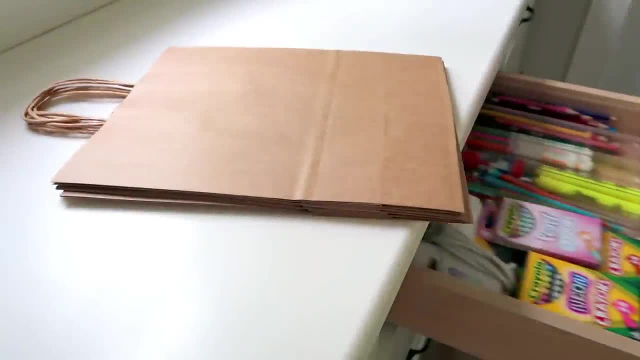 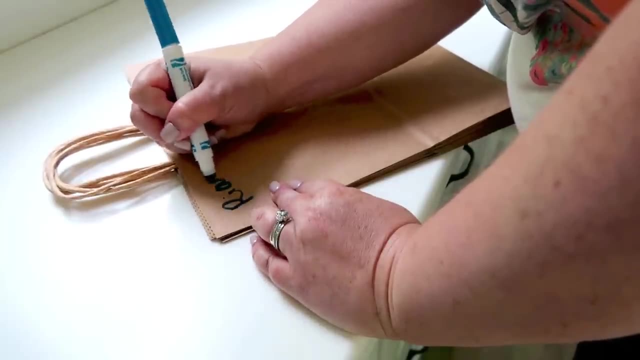 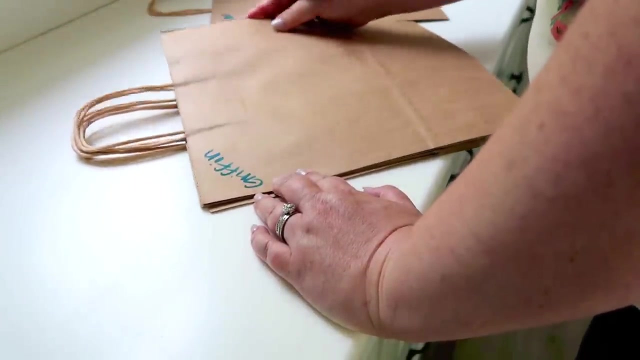 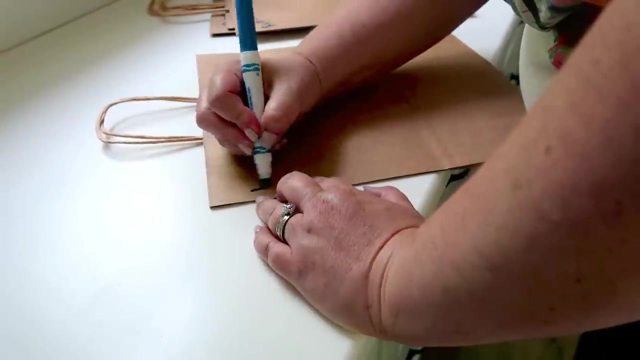 And here is the final look at the supply drawer. I love how this turned out. There is nothing more satisfying than a bunch of back to school supplies all neatly organized in a drawer. We're ready. We're ready for your school year. Let's bring it on. 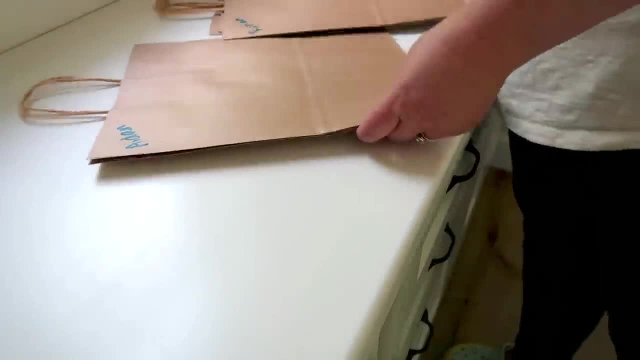 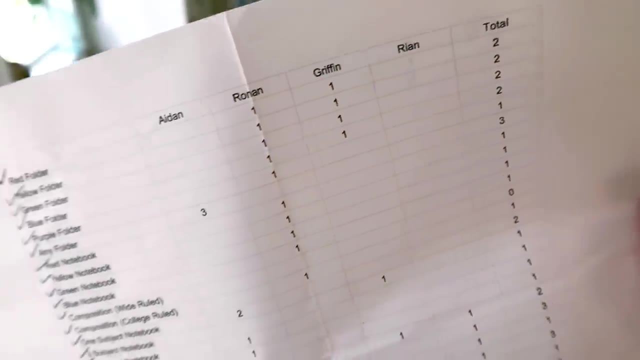 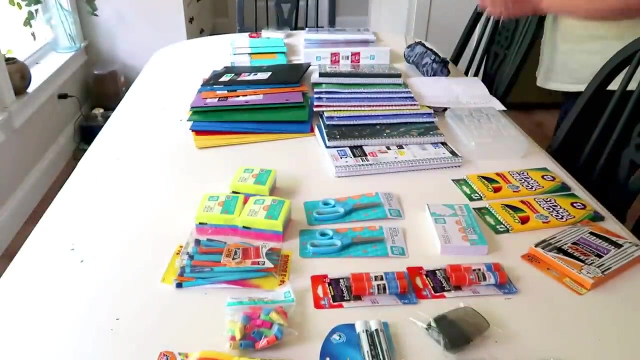 And here is the final look at the supply drawer. I love how this turned out. There is nothing more satisfying than a bunch of back to school supplies all neatly organized in a drawer. We're ready. We're ready for your school year. Let's bring it on. 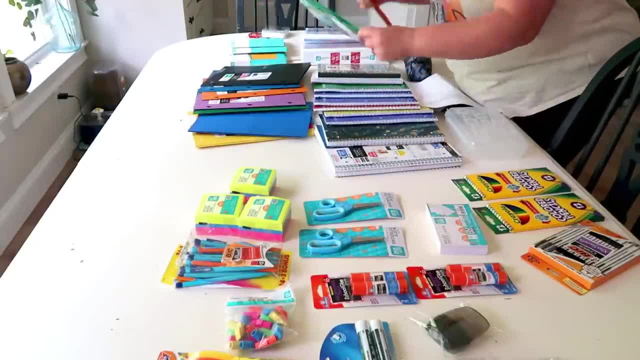 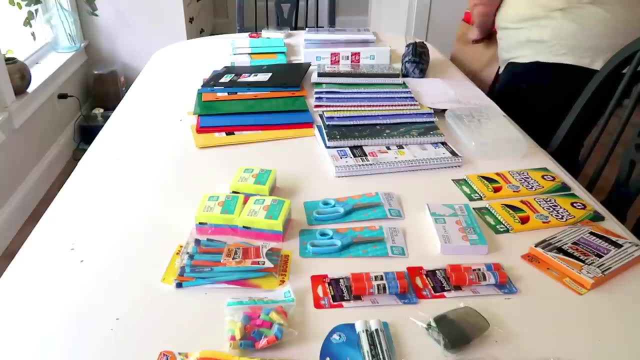 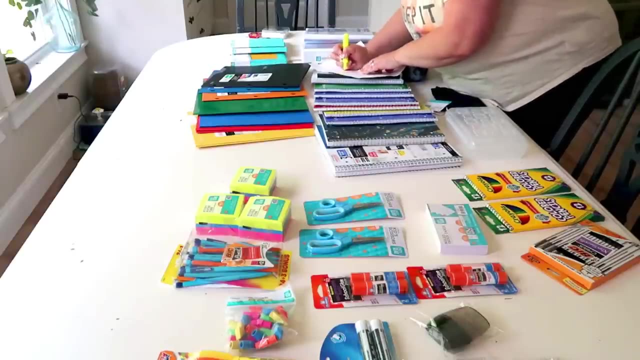 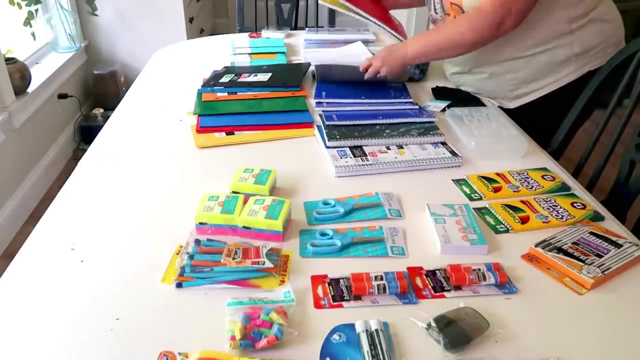 And here is the final look at the supply drawer. I love how this turned out. There is nothing more satisfying than a bunch of back to school supplies all neatly organized in a drawer. We're ready for your school year. Let's bring it on. 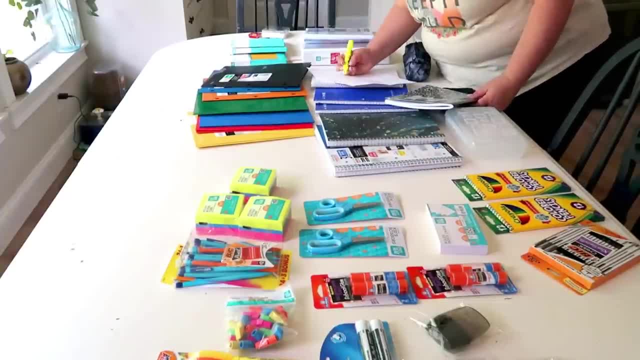 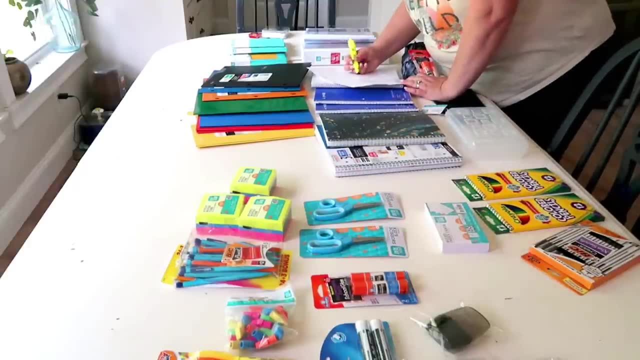 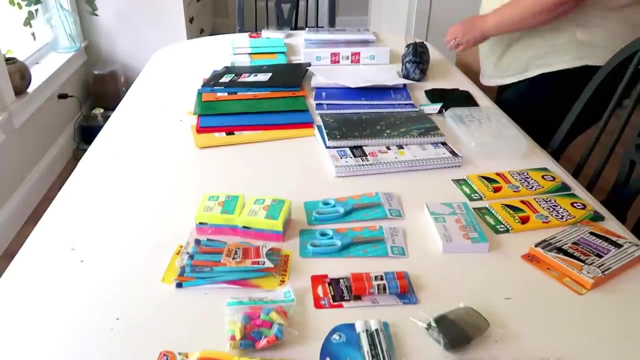 And here is the final look at the supply drawer. I love how this turned out. There is nothing more satisfying than a bunch of back to school supplies all neatly organized in a drawer. We're ready for your school year. Let's bring it on. 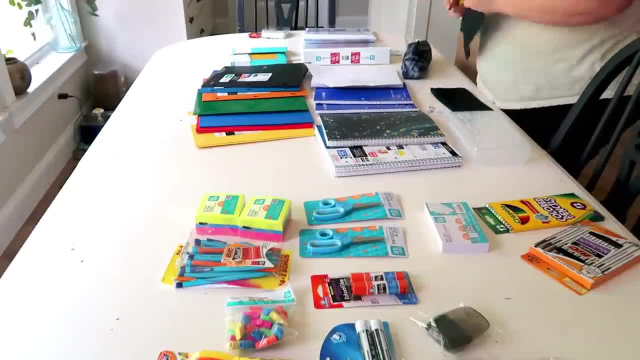 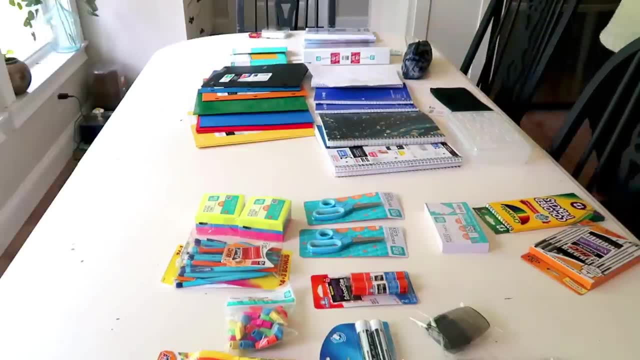 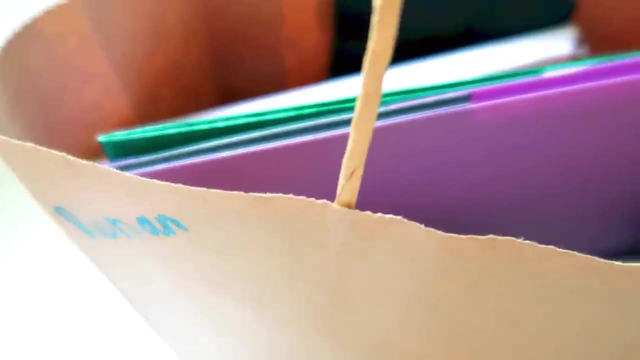 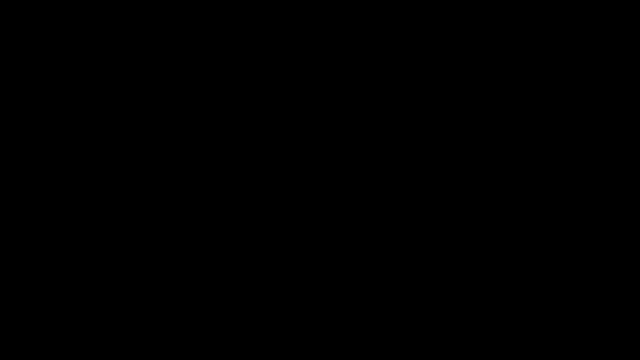 And here is the final look at the supply drawer. I love how this turned out. There is nothing more satisfying than a bunch of back to school supplies all neatly organized in a drawer. We're ready for your school year. Let's bring it on. 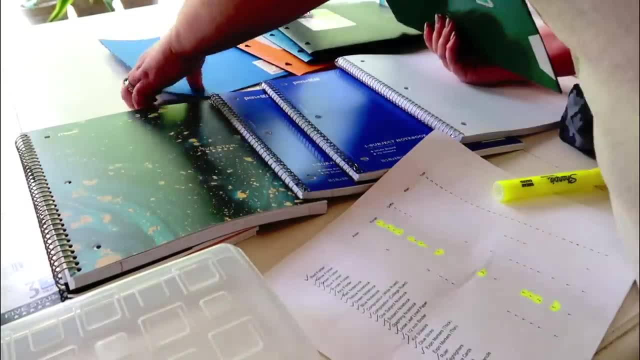 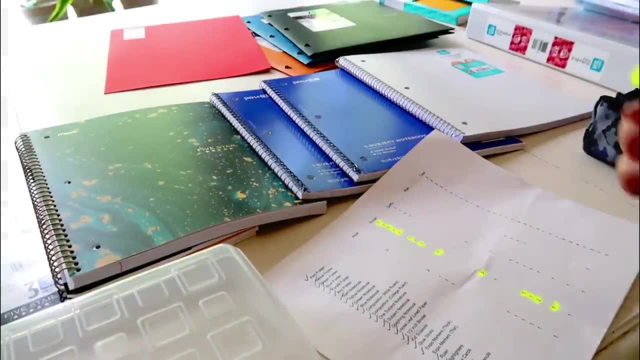 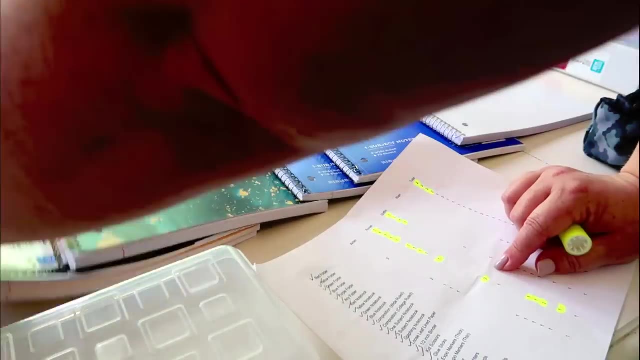 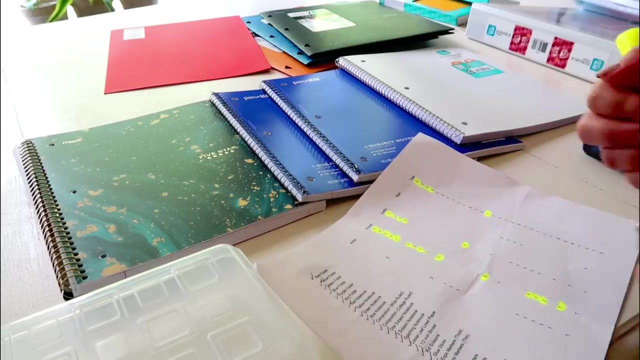 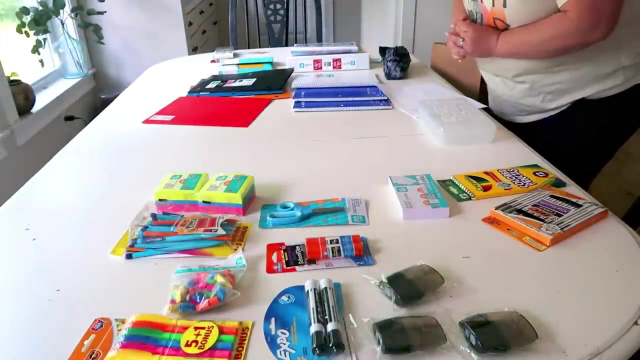 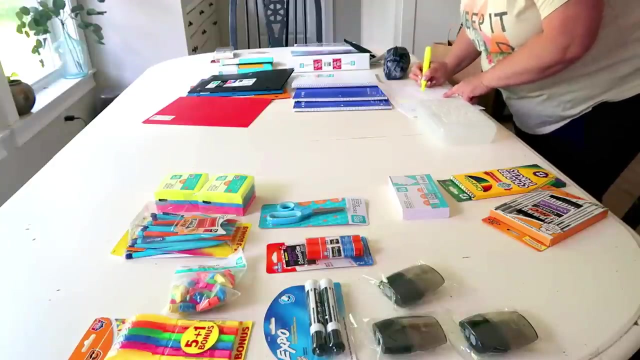 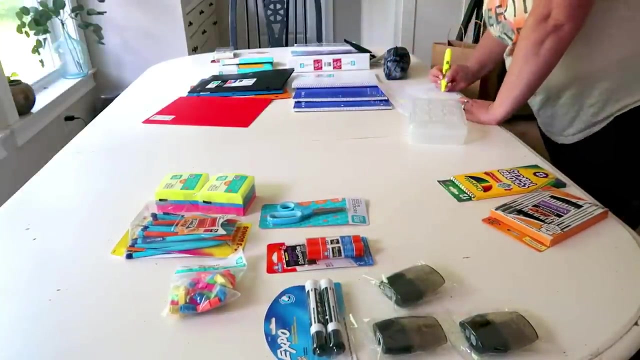 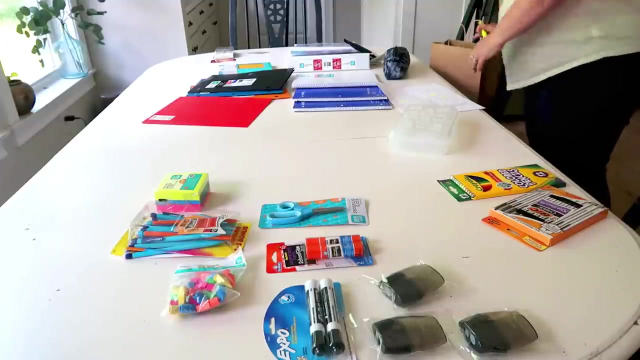 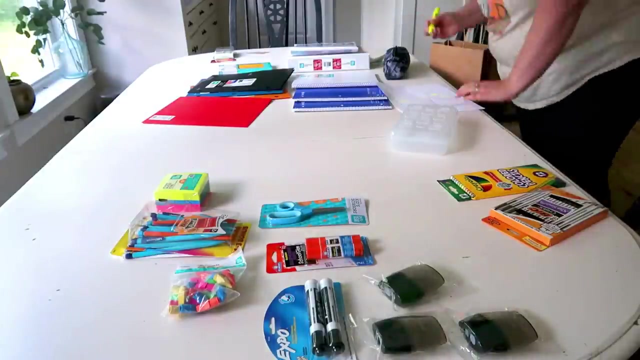 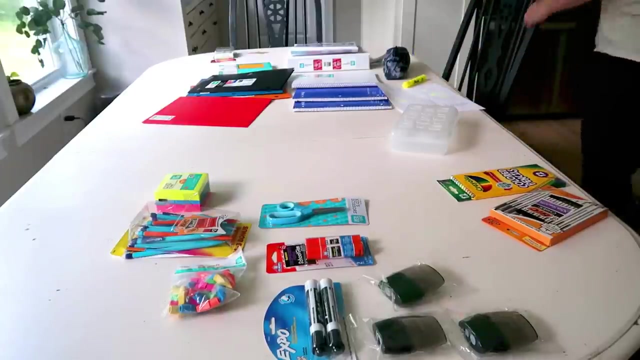 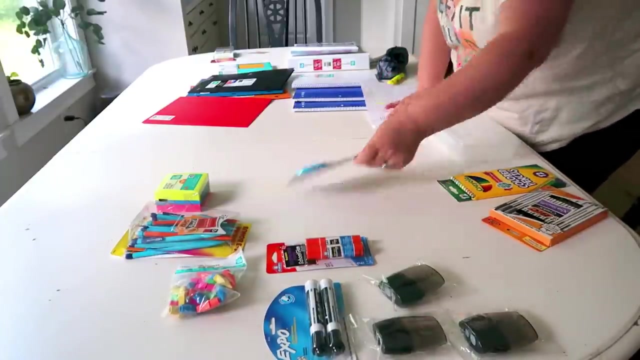 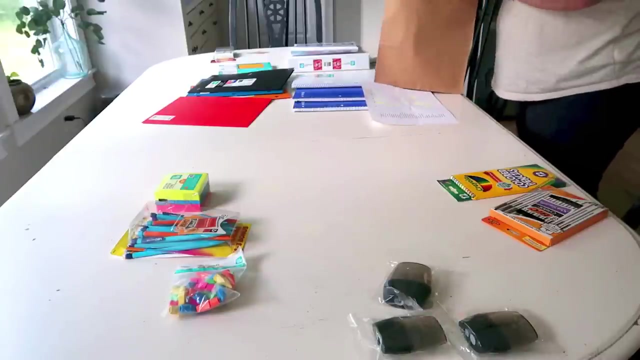 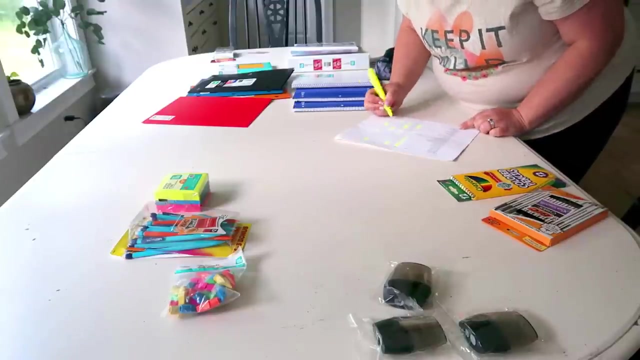 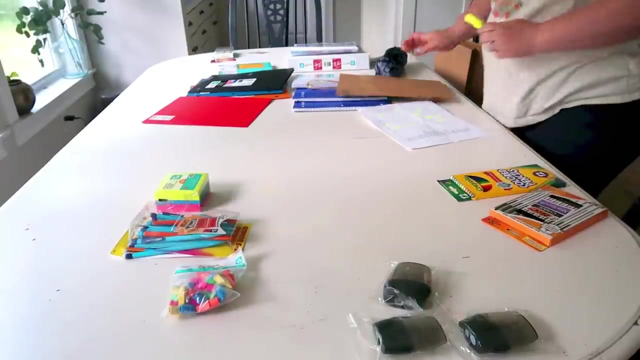 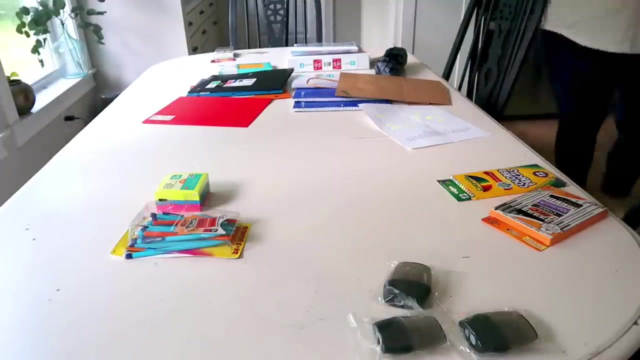 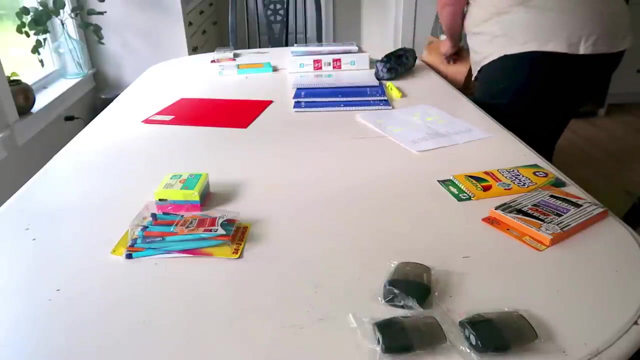 This will be highlighted and all the supplies will be in bags. And here is the final look at the supply drawer. I love how this turned out. Let's bring it on. This will be highlighted and all the supplies will be in bags. And here is the final look at the supply drawer. I love how this turned out. There is nothing more satisfying than a bunch of back to school supplies. 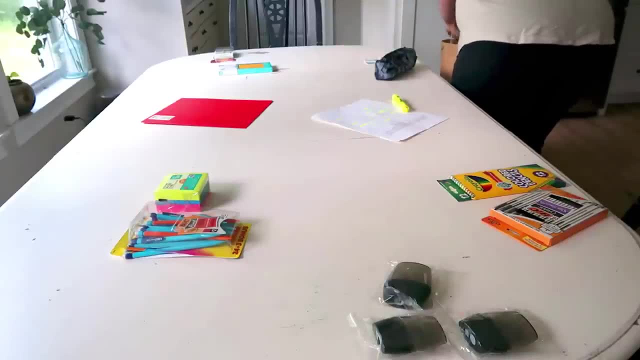 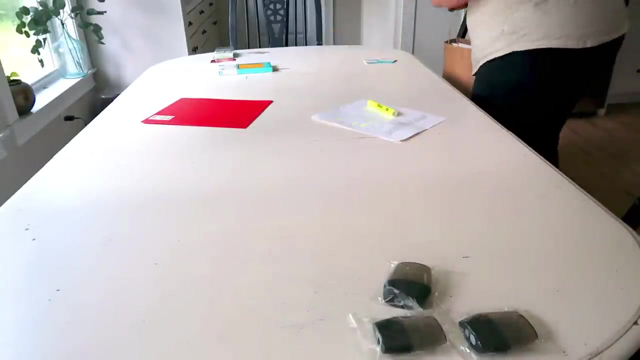 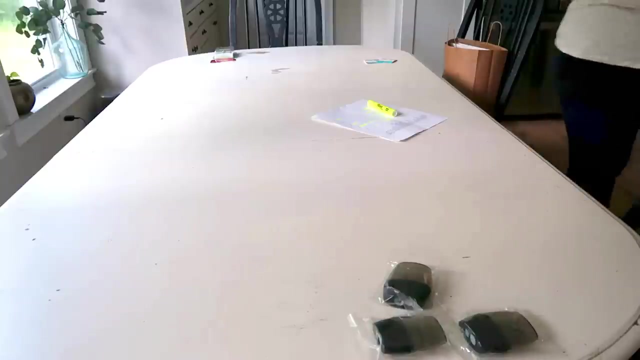